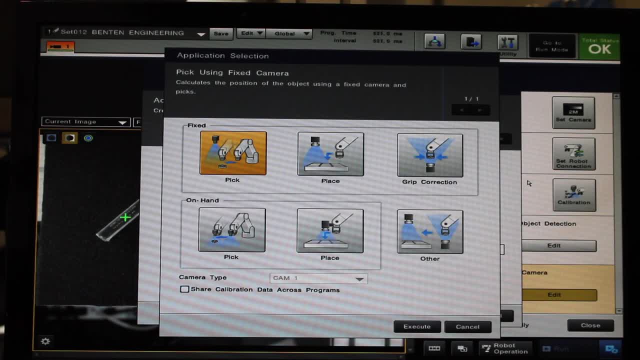 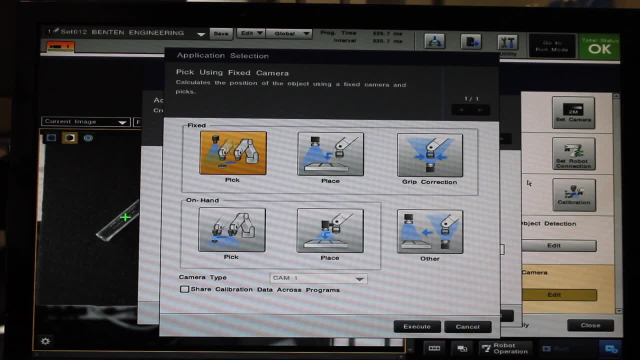 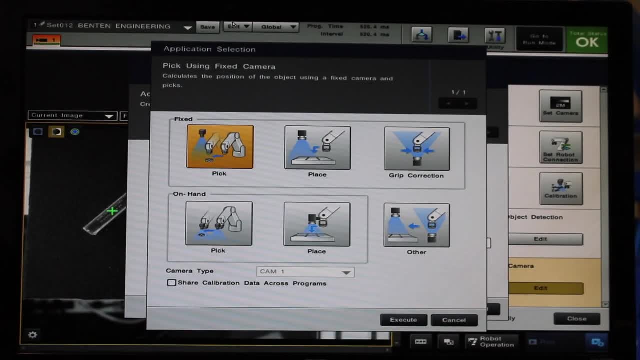 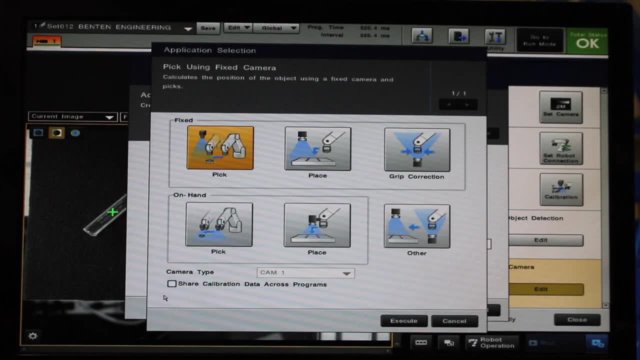 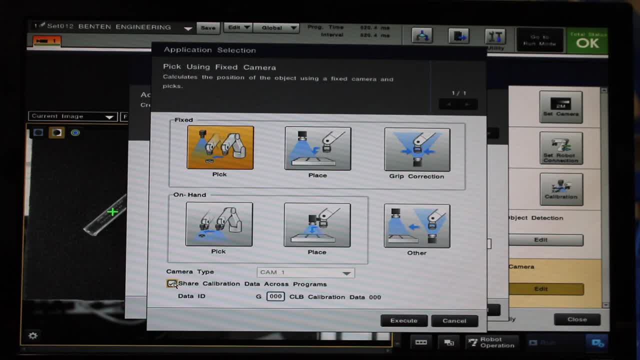 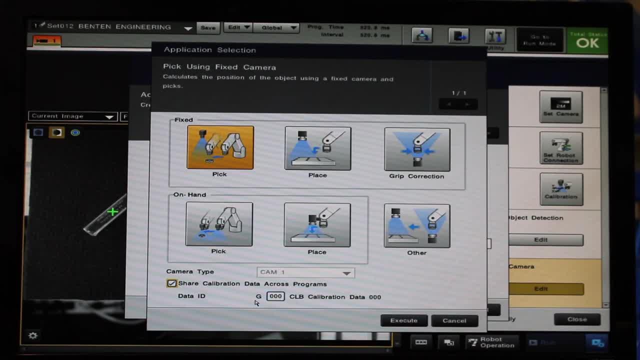 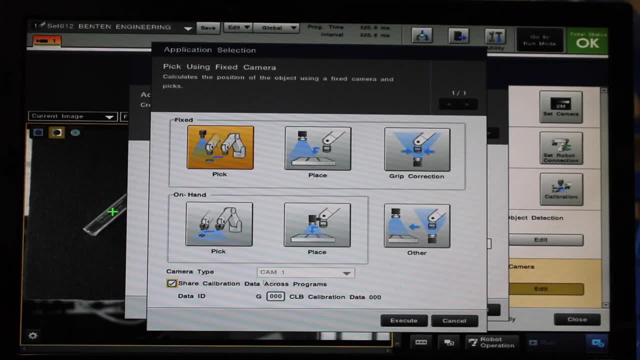 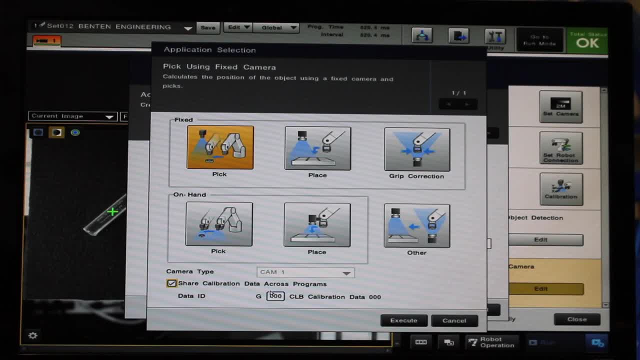 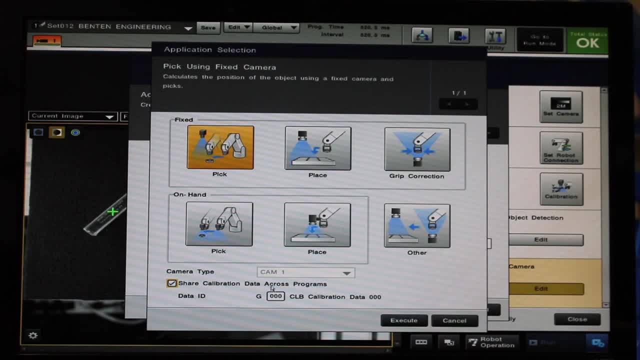 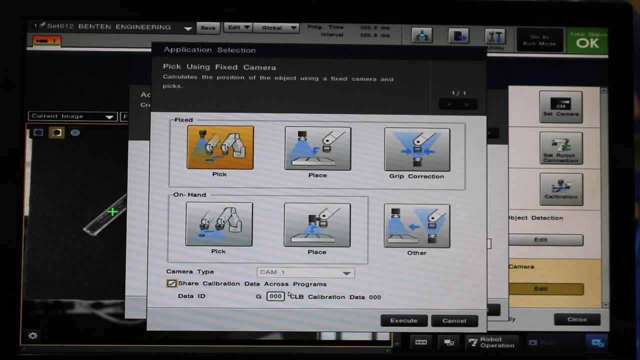 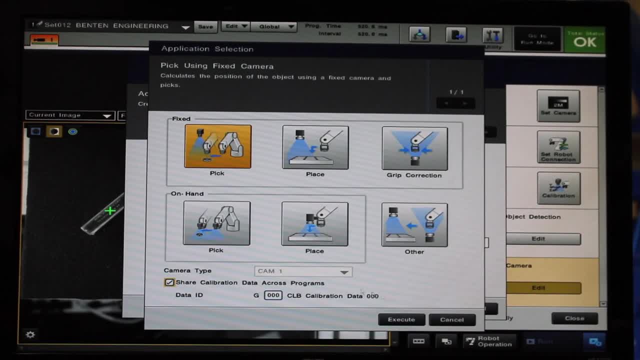 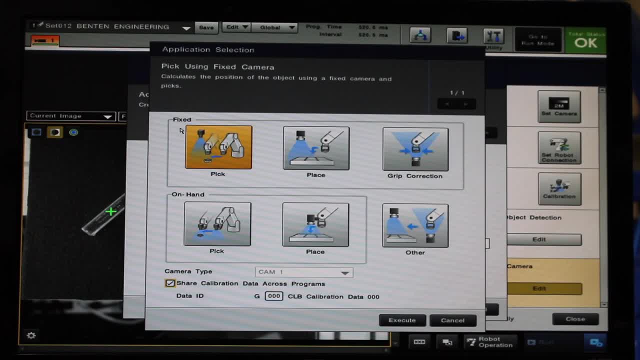 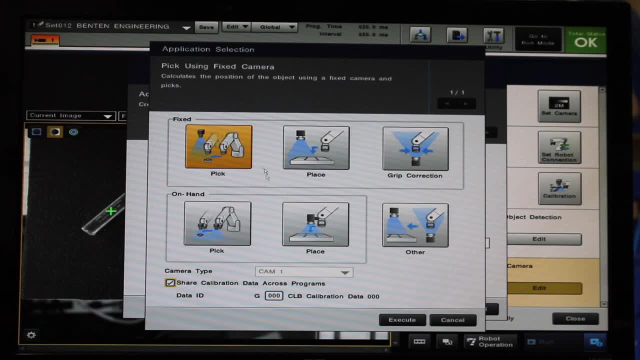 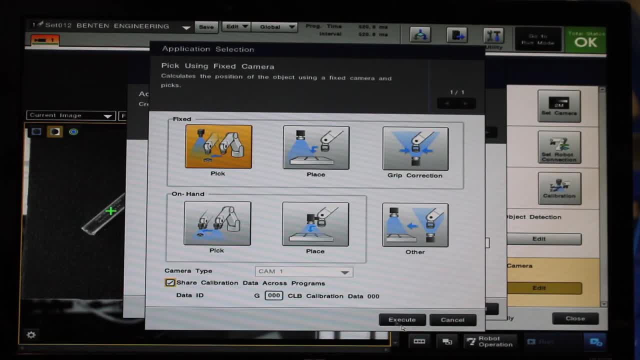 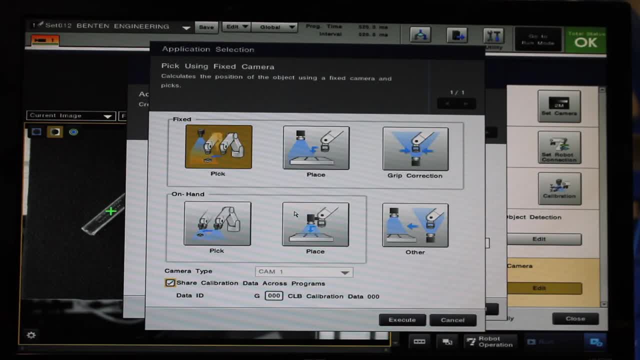 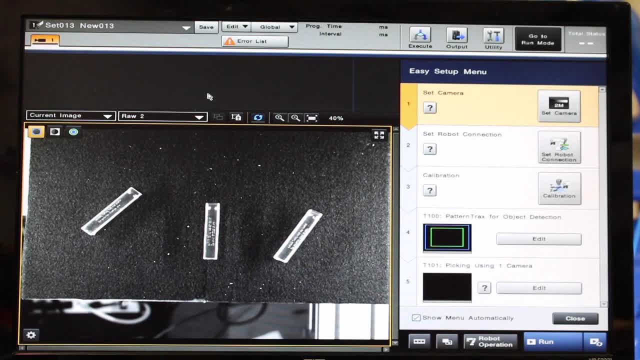 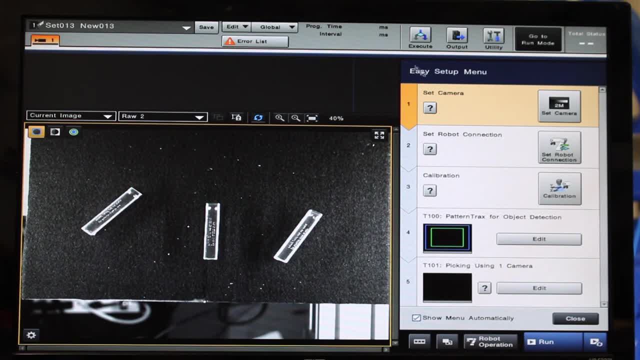 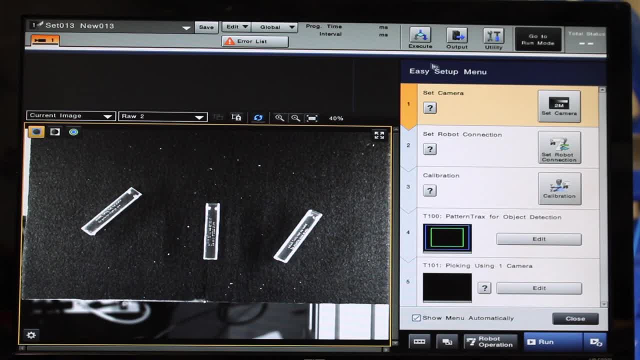 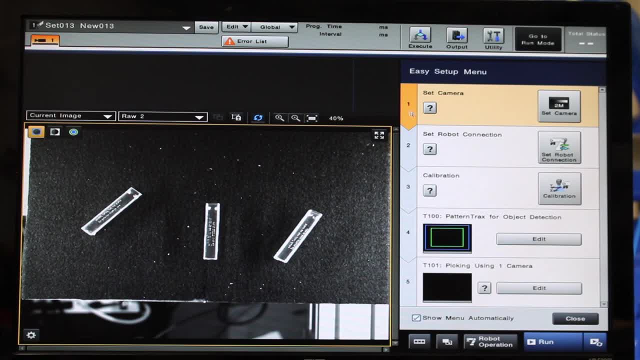 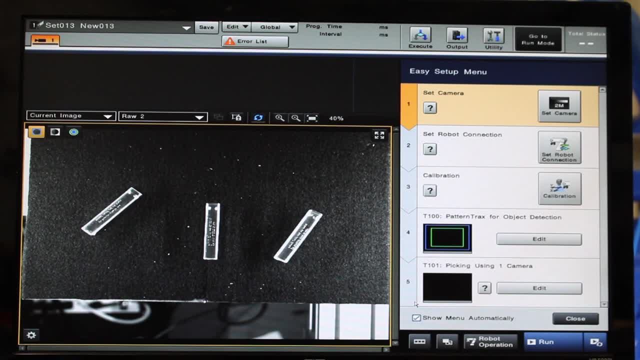 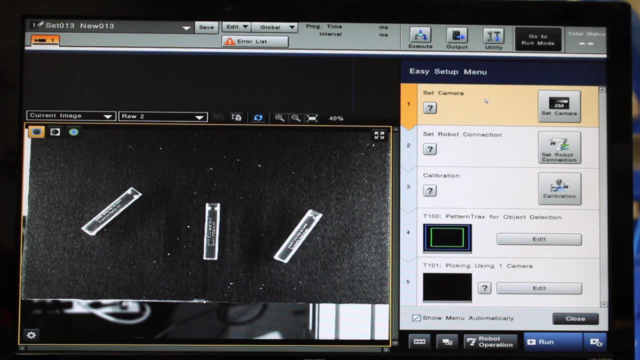 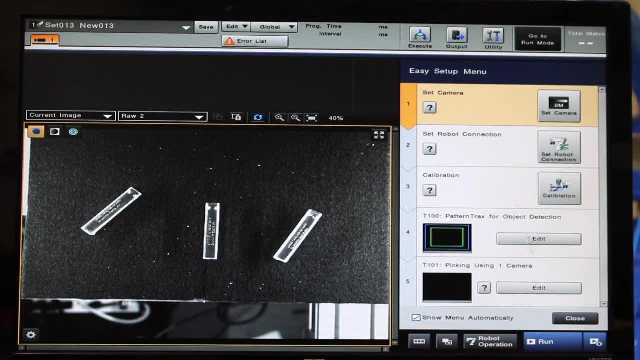 I am here to show you one of the many questions I have been asked. I am here to show you one of the many questions I have been asked autonomously. pick your part. So the first step we have here is setting the camera: The camera. 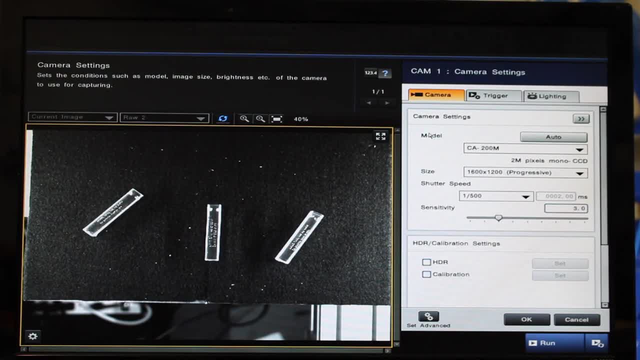 that we're going to be using and the camera settings as well. So it should automatically pick up the model camera you're using if you are connected. Right now we're using a CA200M. As far as the size goes, we don't touch that. You can play around with it. It does change a. 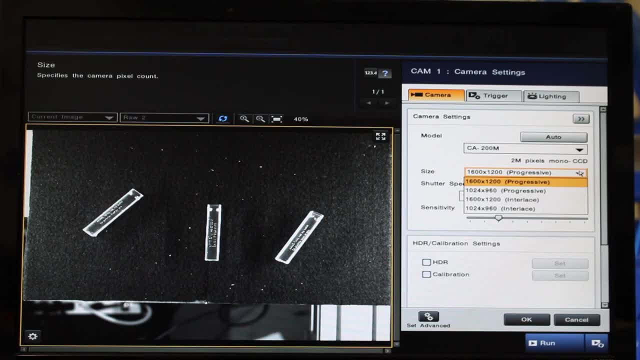 few things, but we have it on 1600 by 1200 progressive, So we're going to leave it where it is. As far as the shutter speed goes, the shutter speed is what is allowing light into the camera, how much light is being allowed in, And so right now we're set to 1500.. And you can. 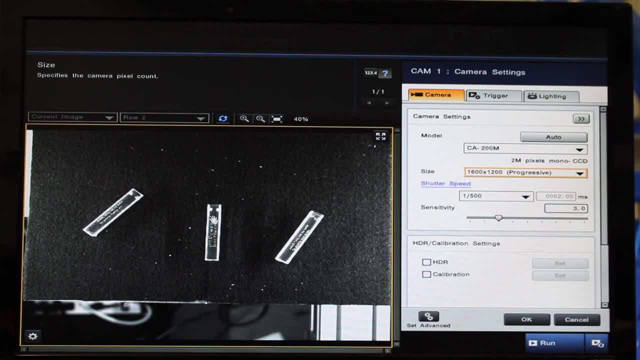 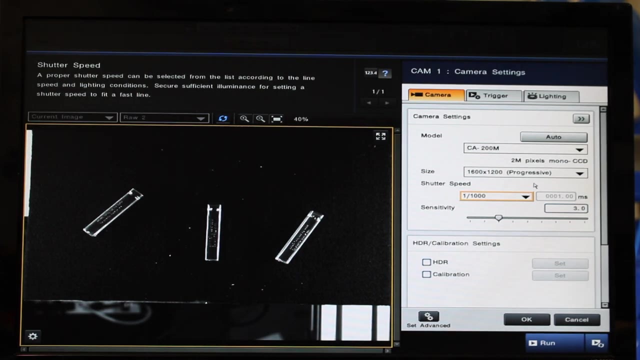 see the three pieces, the three parts we have currently in our field of view. They are pretty bright and you can see them pretty well, And what we can do is if we were to raise this up to 1100, you could see the picture instantly gets darker And so, depending on the part that you need picked, 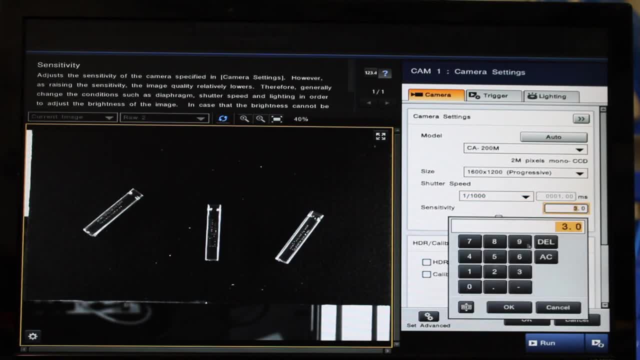 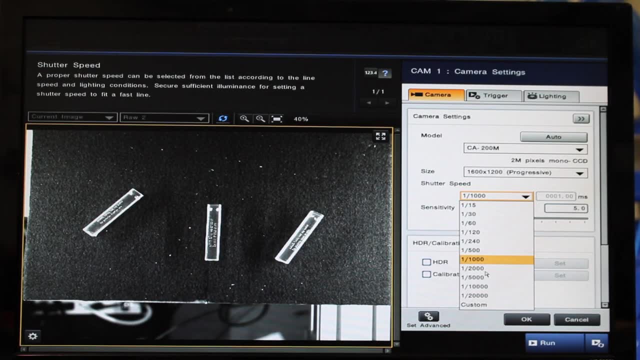 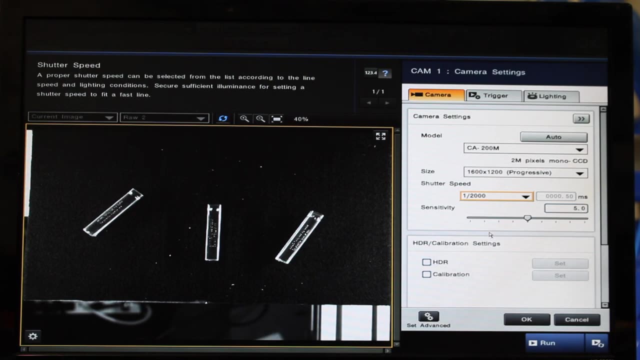 you can play around. You can play around with this as much as you want. You can also play with the sensitivity here. Raising the sensitivity will allow more light in, whereas raising or lowering the shutter speed will allow less light in. So you can play with that to your heart's content And depending on. 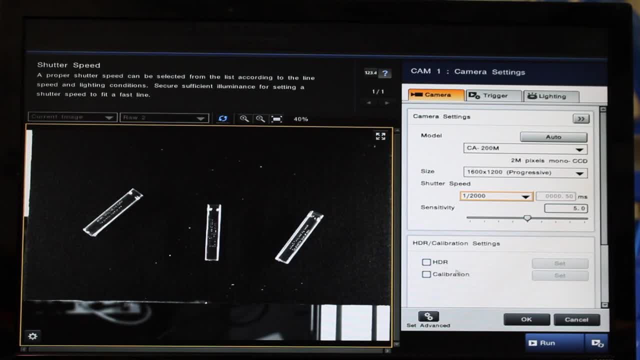 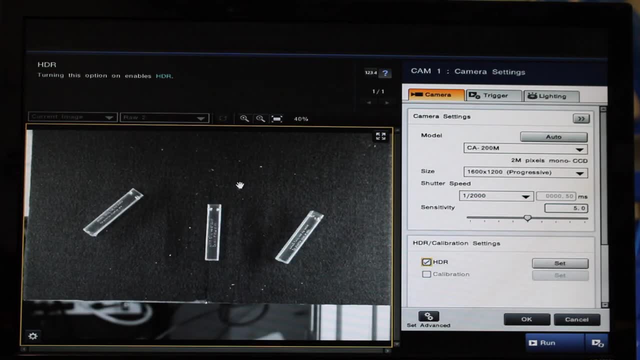 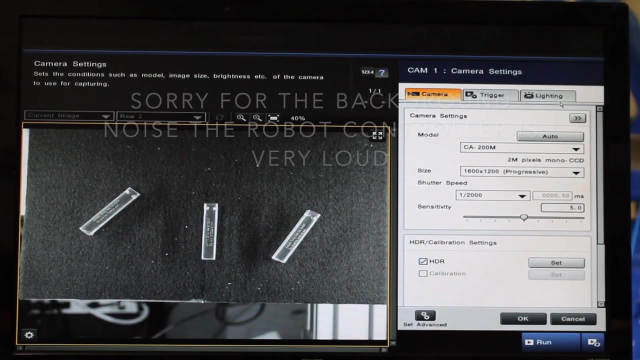 the circumstances needed. you can mess around with that. The one thing that we do want to add, though, is HDR. Once we check this, we get a much cleaner, more monochromatic image, which allows for better feature extraction. Okay, so, once we are done actually setting up the settings for the camera and getting a good image, 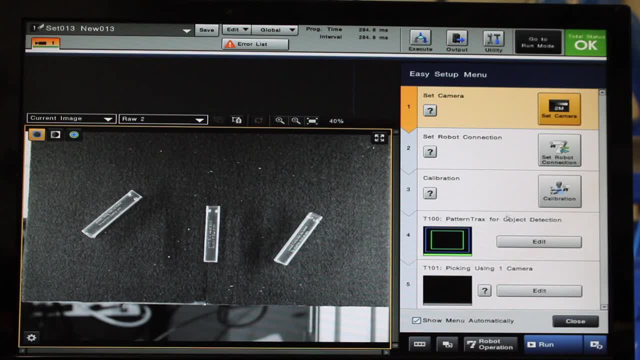 that we want and we're okay with, we can click okay, And the next step, step two, would be to set the robot connection. We want to make sure that the arm that we're using is properly connected to the vision controller and that they can communicate with one another, So if we click over, 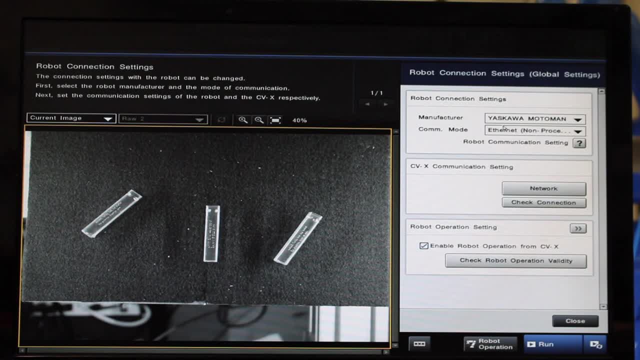 here set robot connection. you can see the manufacturer we have set is Yaskawa, because we are using a Yaskawa arm And our communication mode is ethernet. We have an ethernet cable connecting the arm to the vision controller And if you have an ethernet cable connecting them, 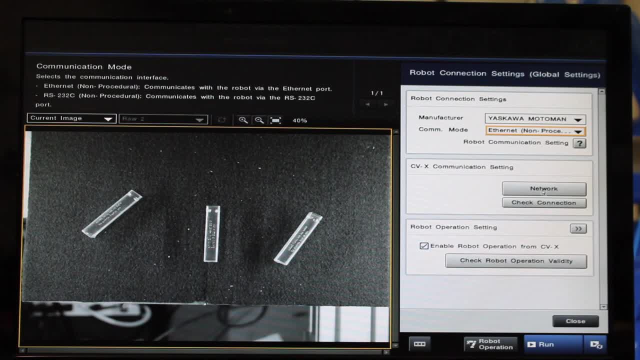 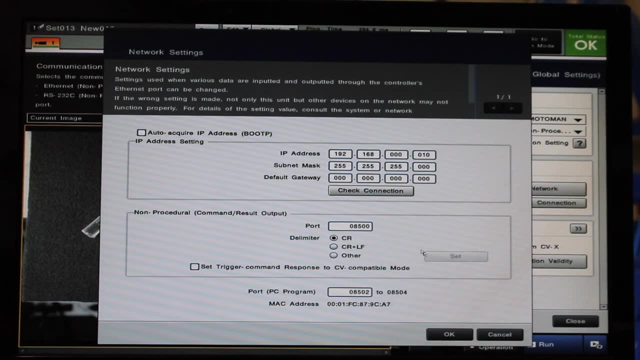 and we head down here to the CVX communication settings. these network settings should be automatically populated once you are actually connected. If not, you'll want to find out this, this information. So that's it. Thanks for watching. See you next time. Bye. 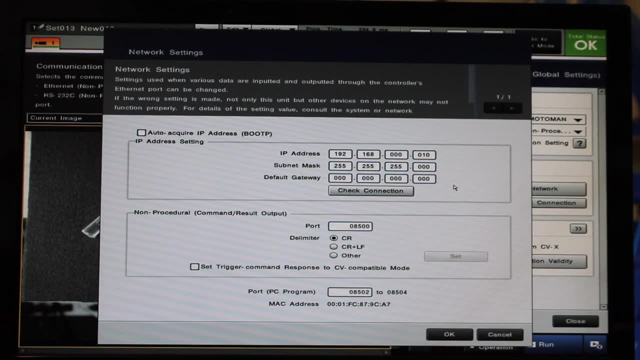 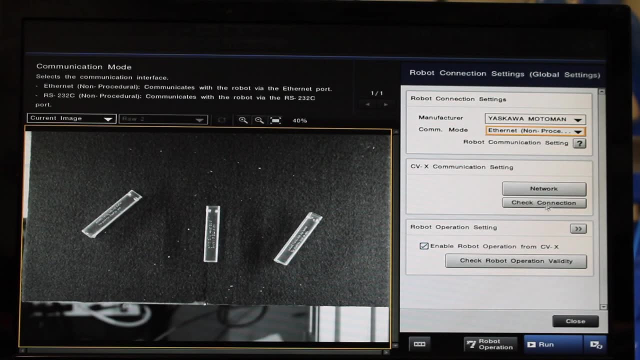 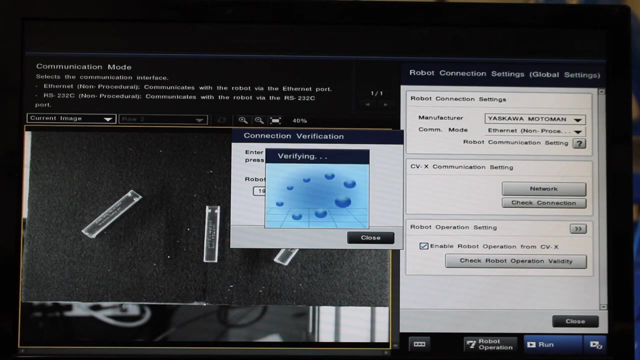 So we'll click okay there And the first thing we're going to do is right under network there's a check connection. We're going to check the connection and we'll put in the robot's IP address and we're going to ping it. We're going to make sure that they're able to talk to one. 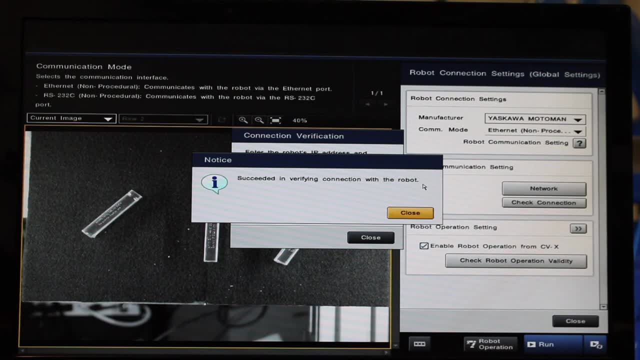 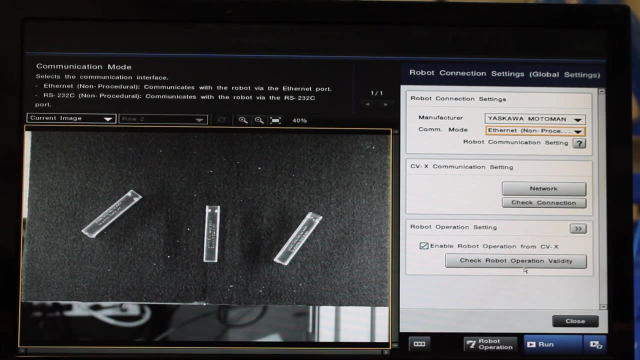 another. So it succeeded in verifying the connection with the robot, which is great. We'll close that out. And then the next thing we want to do is we want to check the robot operation validity With this. we're going to check the robot operation validity With this. 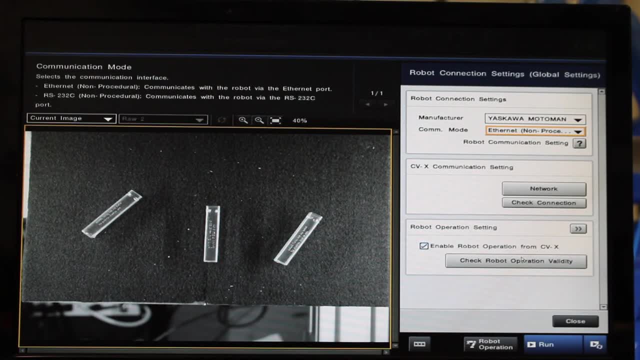 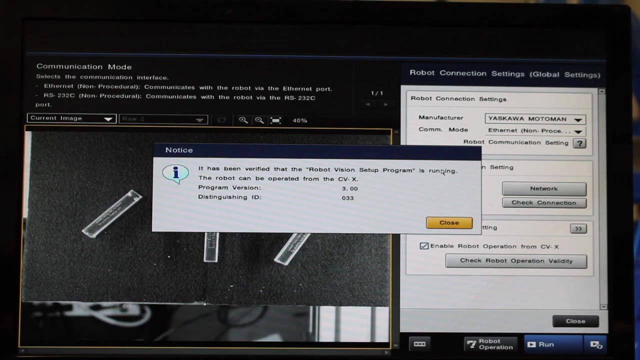 we'll allow us to do is actually operate the arm through the program here, the vision program. If you can see, down here there is a little robot operation button. So once we check the operational validity which it has been verified, that the setup. 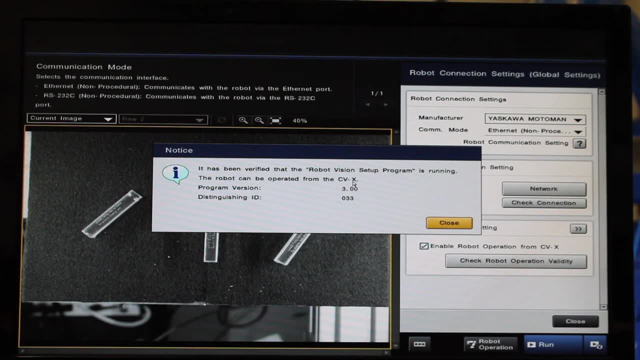 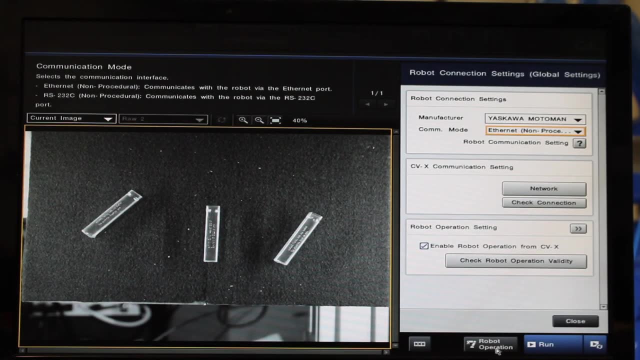 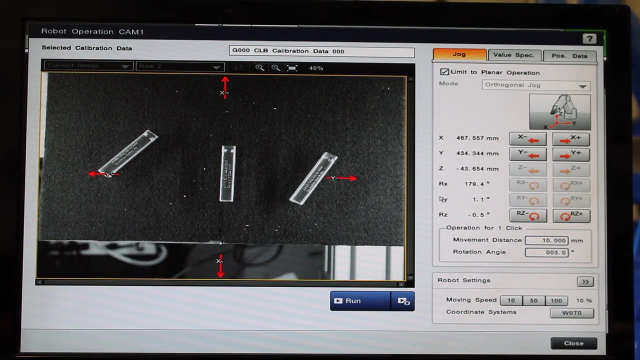 program is running and it can be operated from the CVX, which is our vision controller. So once we have confirmed that that is operational, we can go down here to robot operations And, as you can see, we have our XYZ and our rotational XYZ So we can fully operate the arm using the program. We can move it in the XYZ whichever way we want it to move. We can change the moving speed and the coordinate system that we're using. 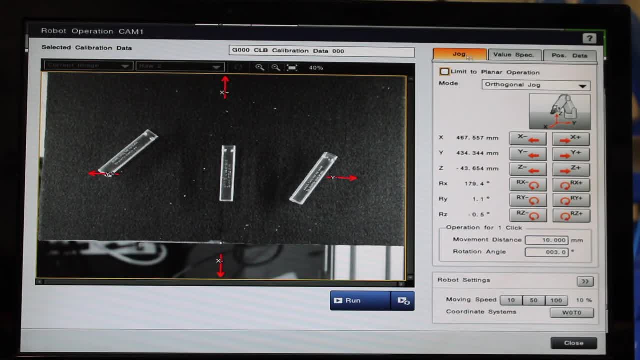 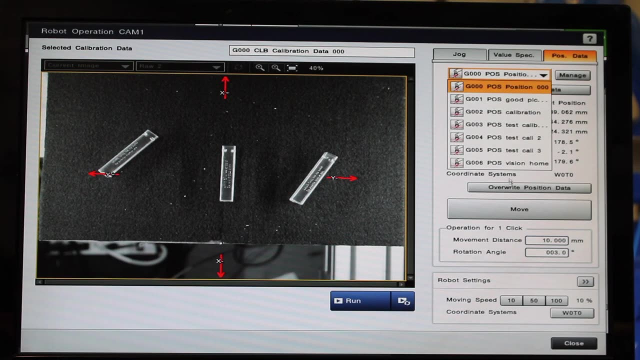 Now, the one thing that I do want to note is up here the three tabs we have: jog, value specifications and position data. Jog is to operate the robot manually. Position data is very important, at least in my opinion. We can set different positions and we can save those positions. 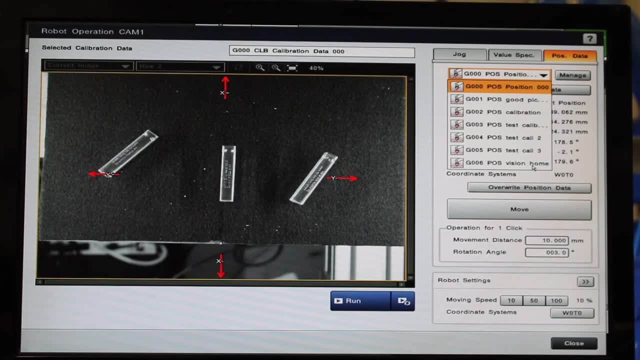 And so if we let's say vision home- I already have one set called vision home- If we move the robot to a certain position, we can save that position And we don't want it there anymore. Instead of manually having to move it back, we can simply set, we can simply turn on vision home and then click and hold, move and it will continue and it will move to that position. 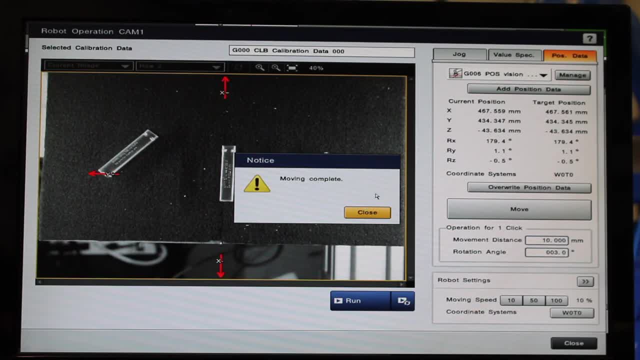 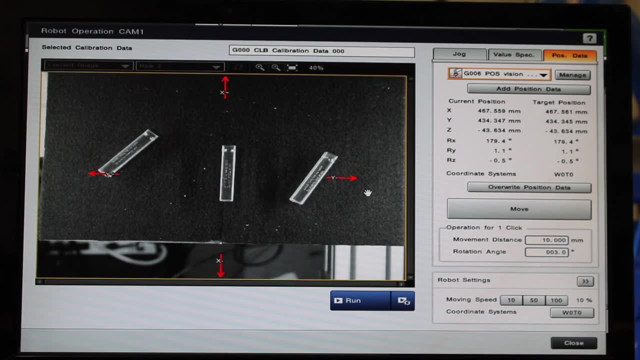 Now, since the robot is currently in that position, it says move and complete the second. I press it, But if you press and hold, you can move the robot to that position or whichever position you have it set to. The next step we're going to be working on here is actually calibrating the system. 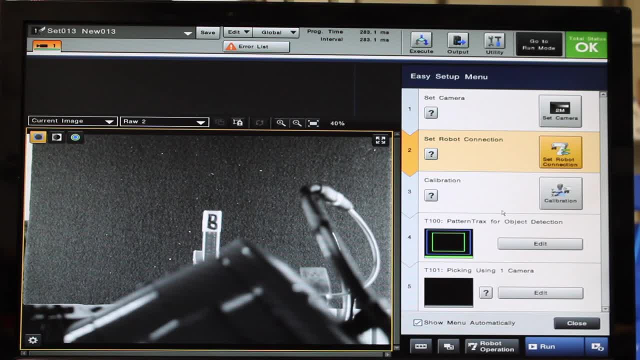 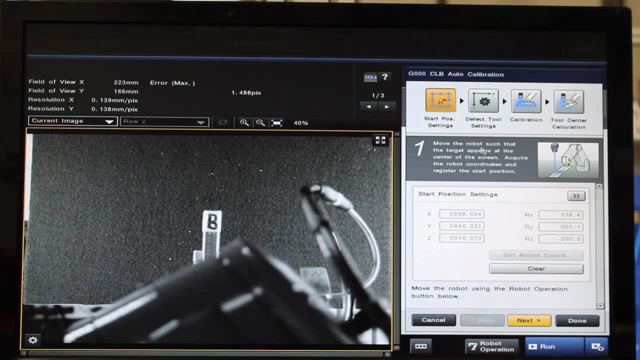 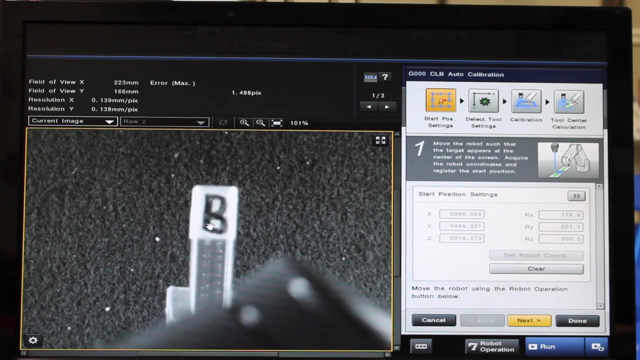 Making sure, Make sure that we have precise picks and the arm knows where it's going and where it can go. So the third step here: calibration. we'll go ahead and click on that and get in there, And so the first thing we're going to want to do is actually, if you can tell, I went ahead and I put a piece of tape with a B for Benton Engineering on here. 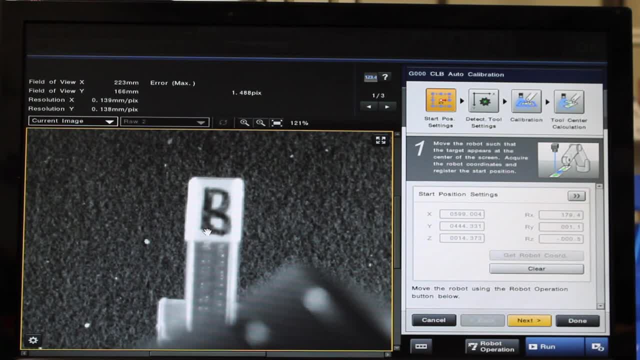 You want to use a dark featured, asymmetrical design, anything. It could be a smiley face, It could be an A, a, B, a lettering numbers, anything that is asymmetrical and very distinguishable. So, as you can see, the vision system has no problem picking this up. 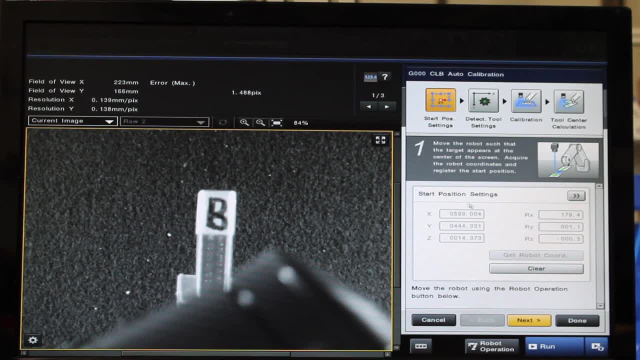 And so the first step that we want to do is we want to get the robot's coordinates or the start position for the calibration. So, whatever position the robot's currently in, you want to have it in the field of view of the camera, which we do. 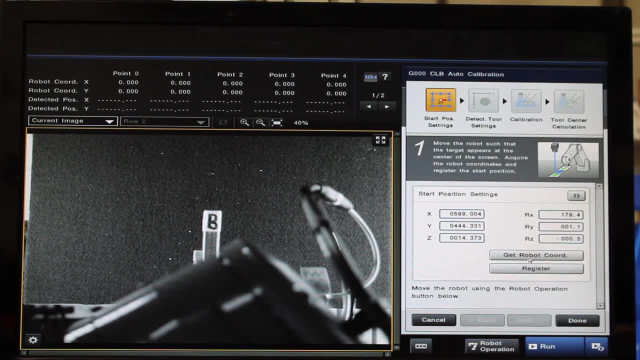 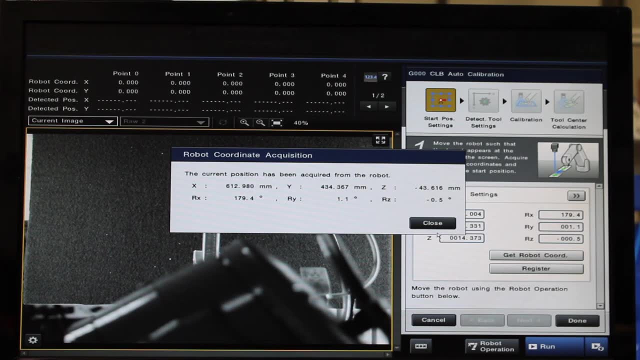 You can see our arm right here, And so what we're going to do is we're going to go ahead and click on that, And so what we're going to do is we're going to get the robot coordinates right here. We'll click that and that will get all our coordinates where it currently is and where it's positioned. 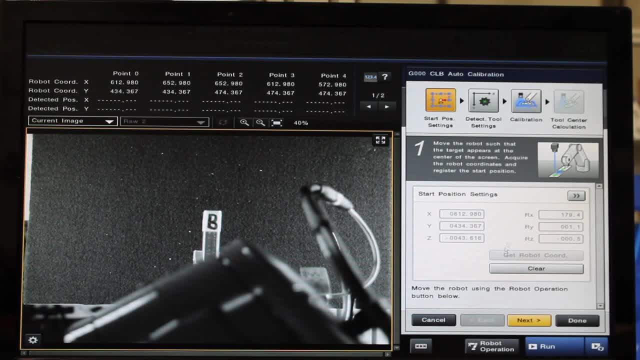 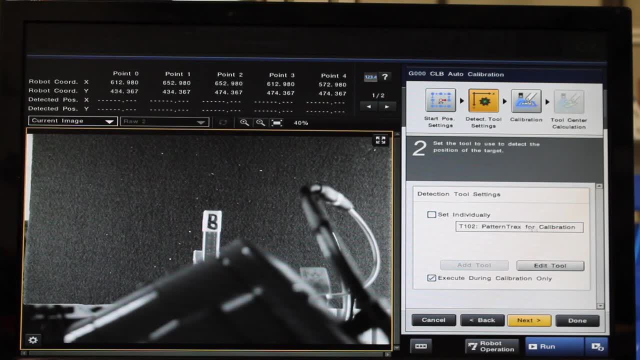 And then we're going to click register. Once we register those robot coordinates, we click next And this is detecting our tool. So you'll see, we're using a Pattern Tracks for calibration. Pattern Tracks is the software tool for identifying specific patterns. 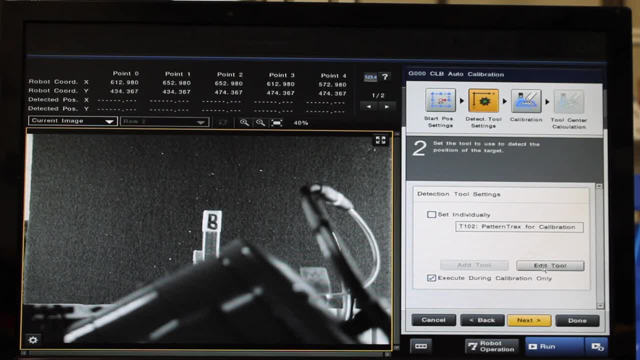 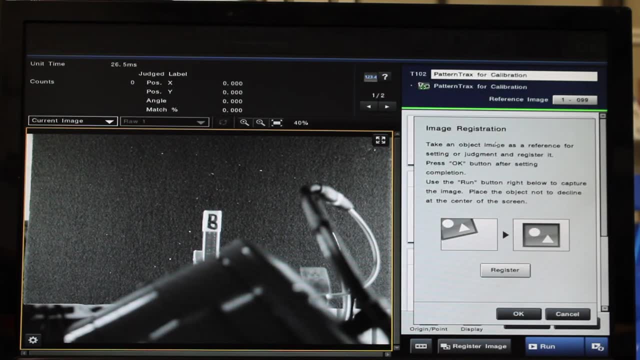 And so we're going to be using that. Right under that you'll see the edit tool button. We're going to go ahead and click edit tool And it's going to ask for an image registration. You simply click register and it'll register the current image on the screen. 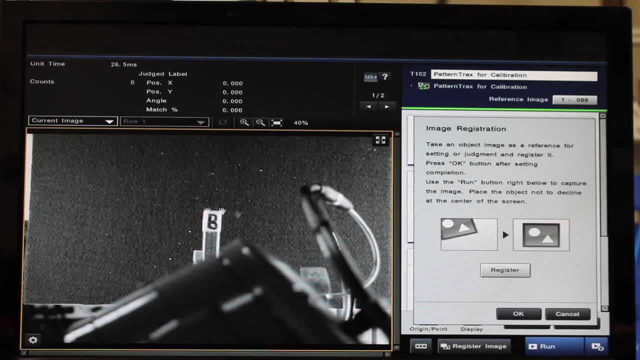 And that's what we want. We want to register this image because this is what it's looking for And keep in mind this is only being used for calibration, So we will go ahead and register that. It'll save that image And then we will click OK. 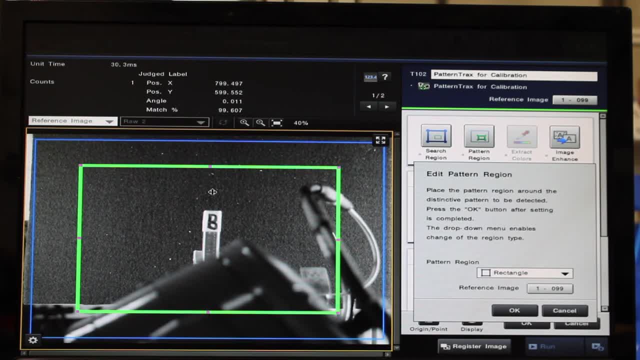 And now what we want to do is: we want to, We want to edit the pattern region, We want to tell the vision system what it's looking for, What specific pattern it's looking for. So, this green rectangle, we're going to go ahead and grab it by the edges. 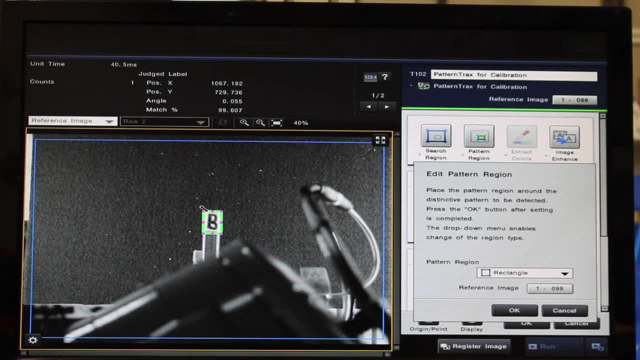 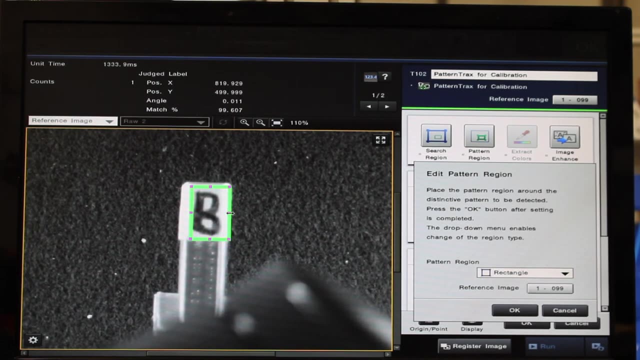 And we're going to surround our B here And try and get it as tight as possible because we don't want it picking up anything else. There we go. So once we have that, you see, I'll zoom in. We have our. 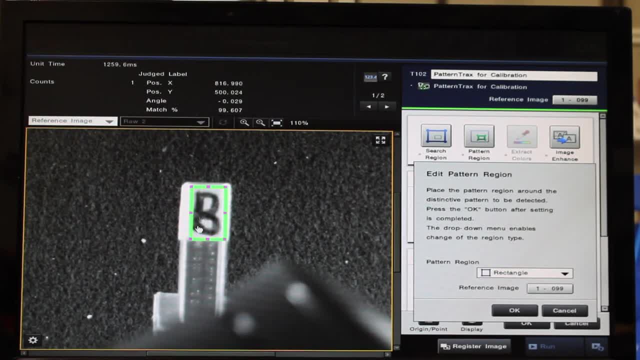 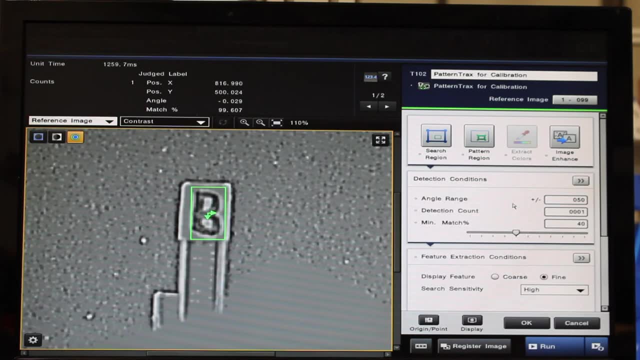 Pattern region around our B. So this is what we're looking for And again, this is only being used for calibration. This is what it's using for the calibration, So we'll click OK here And then you can mess with these settings. 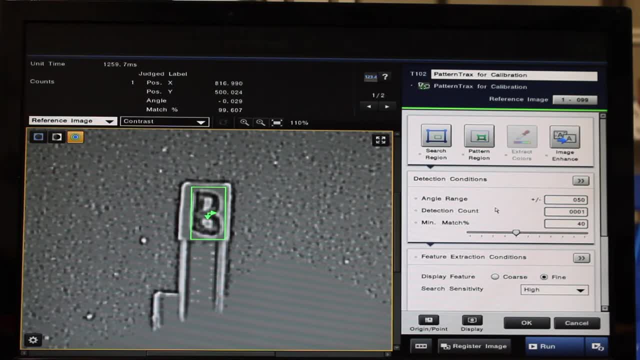 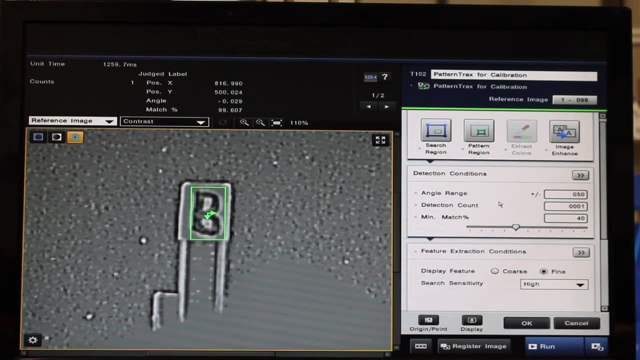 But for calibration, there's no need to. We'll get more into this later on. We'll go more in depth with all these settings, So we'll go ahead and click OK. And so now what we're going to do is we're going to execute. 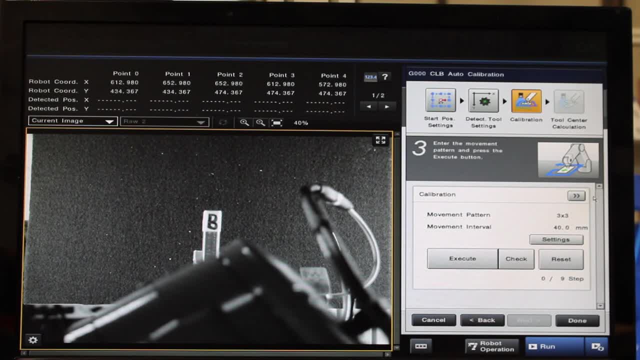 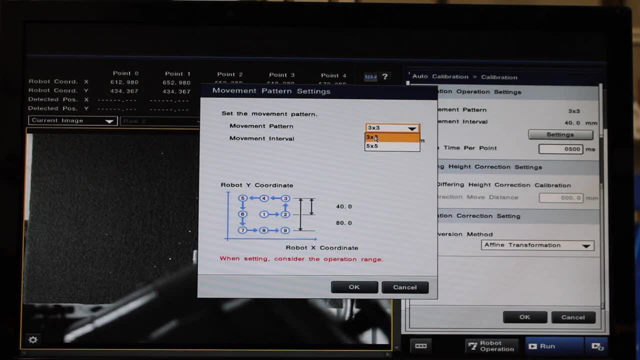 Calibration. So there's multiple movement patterns that you can select. If we go into the calibration settings here, you'll see that I can set my movement pattern for 3x3 or 5x5.. We're going to keep it on 3x3.. 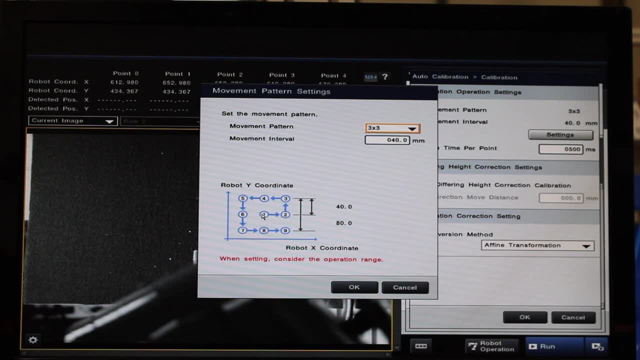 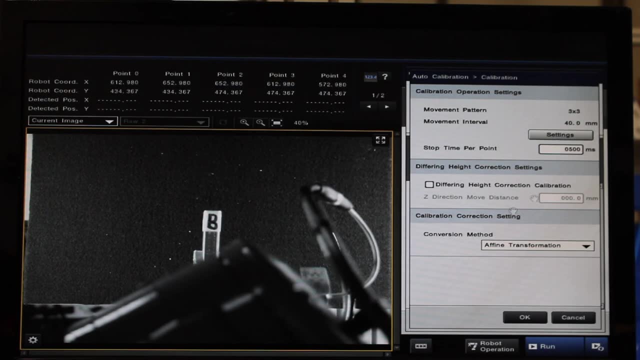 And then the movement interval as well, how far it moves in between each point. I have it set to 40 millimeters. as our space is limited, That can be set to whatever is needed, So we're going to go ahead and set that to 40 millimeters. 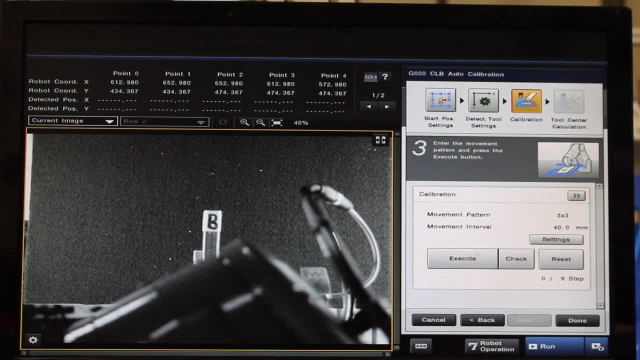 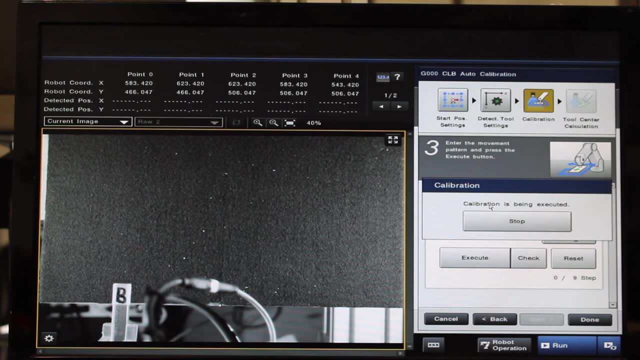 So we're not going to touch anything else, So we'll click OK. Now we just click Execute and we sit and let the system calibrate. So we'll do it completely autonomously. You just have to sit and wait for a little bit and wait for it to finish the calibration. 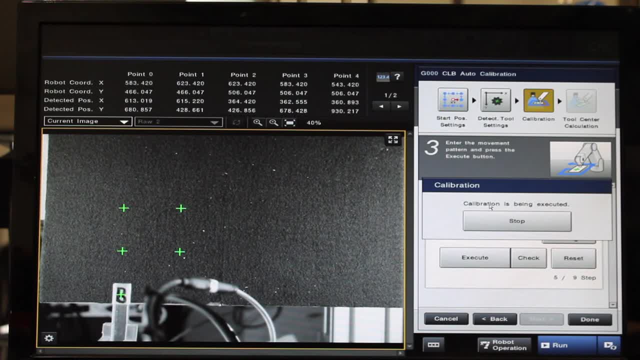 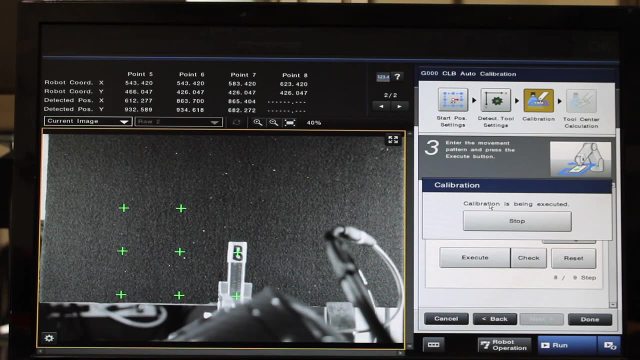 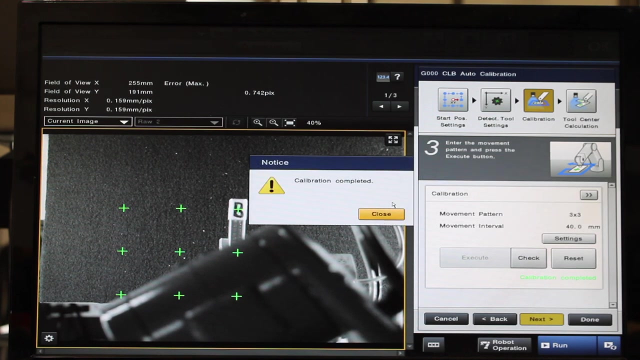 And now that the calibration is complete, you will go ahead and click Next. 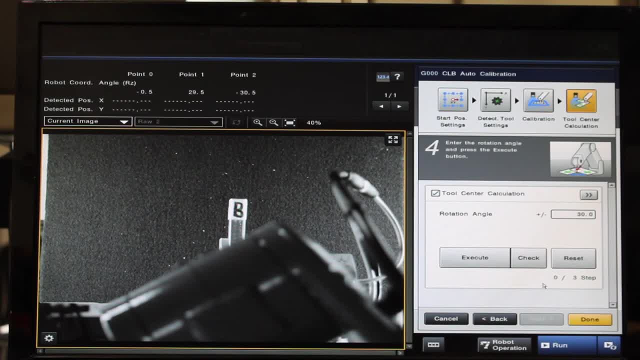 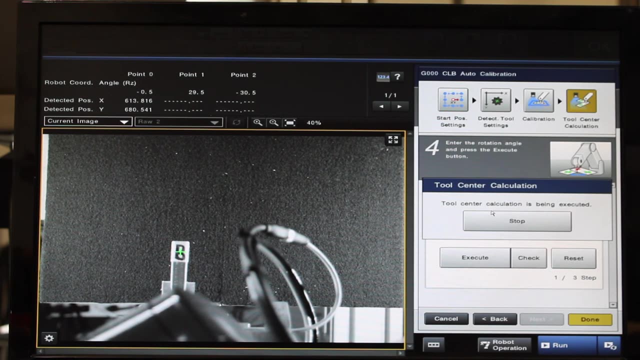 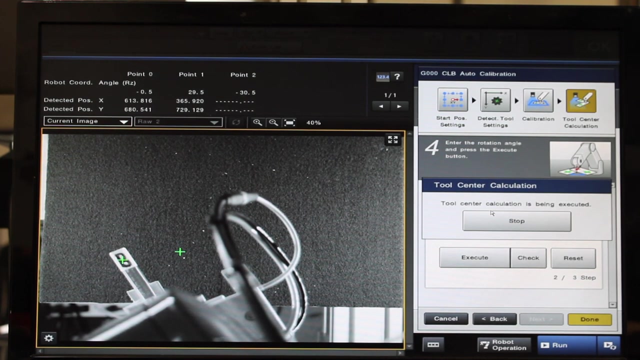 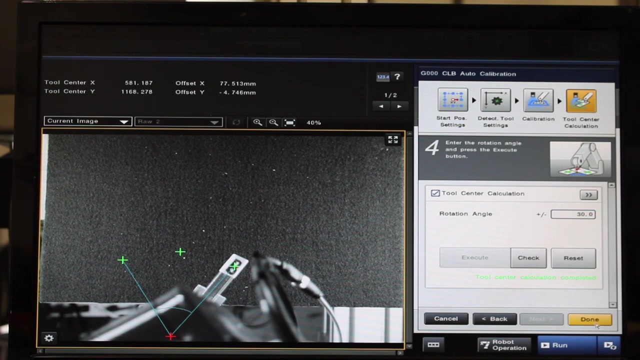 and we'll calculate the tool's center position. And so, once again, we just simply click execute and the system will calculate the center position of the tool, And just like that we have the system calibrated and ready to go. 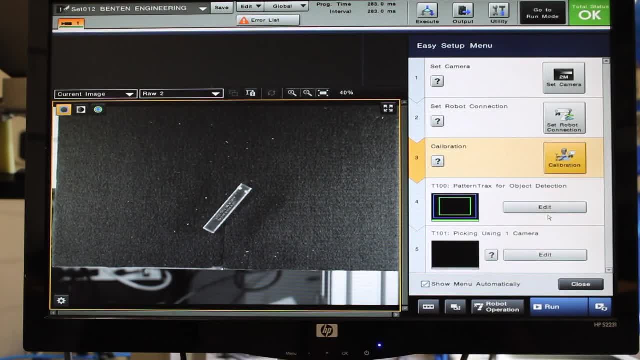 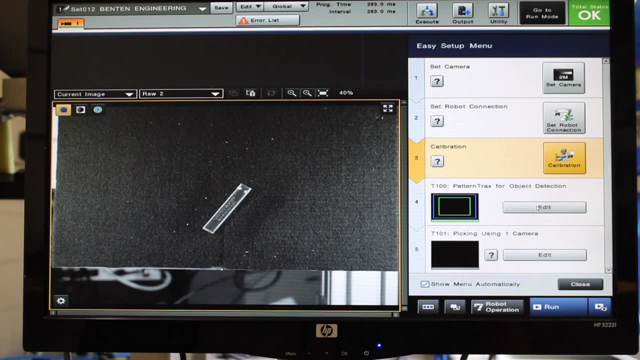 Now we are ready to go into pattern tracks for object detection. We're going to actually be teaching you how to do that. We're going to be teaching the program what is a good pick and what it should be looking for. So right here, step four- pattern tracks for object detection- is what we're looking for. 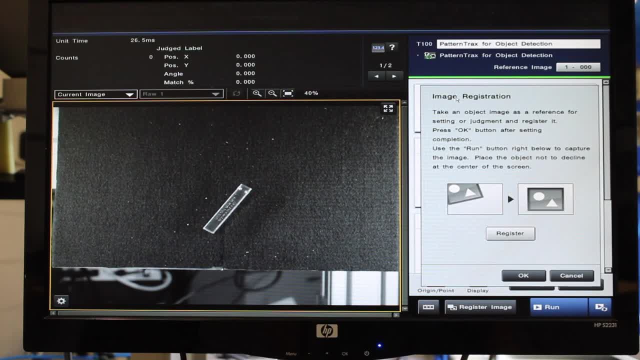 So we'll click edit and that will bring us in, And so you'll see notice right away that it asks for image registration, And so we need to take an image of what a good pick is, so that way it can use that as the reference image. 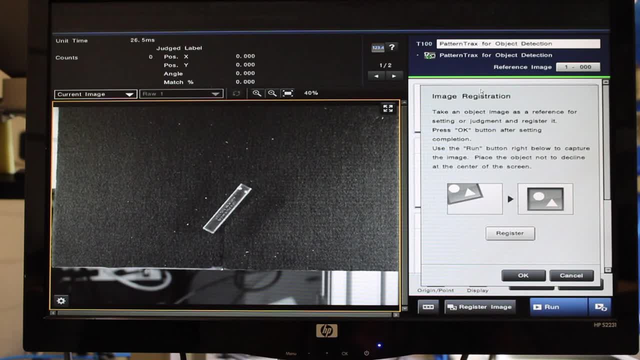 and compare that to any pieces that are on there. So you always want a reference image and we want to teach you what is good, what is not. So what we're going to do. I already set up a piece that we're looking for. 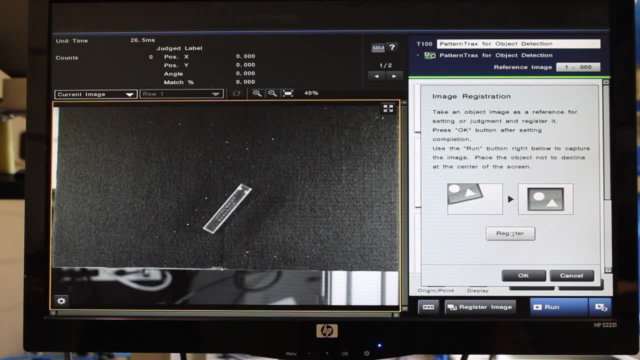 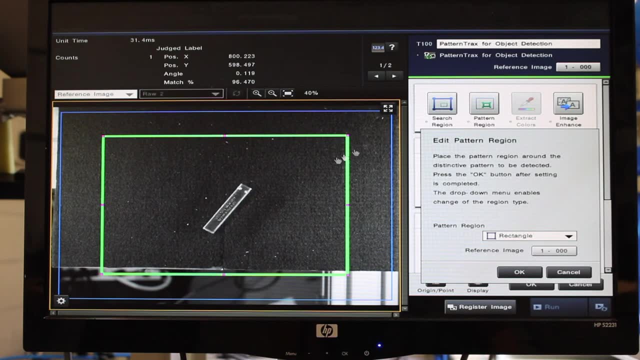 So we're going to register this as our reference image And all we'll click is register and it'll save the image And then we'll click okay. And now it wants us to edit the pattern region. What exactly is it looking for? 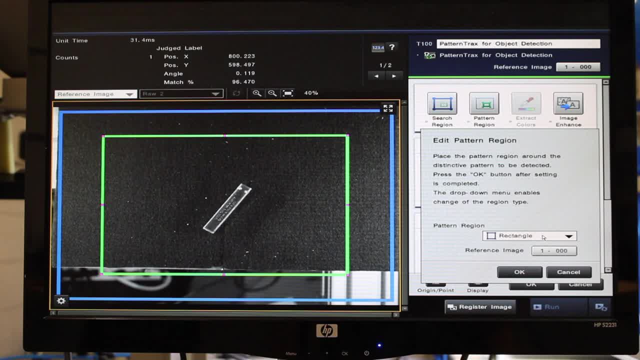 What are we looking for? And so you have a bunch of different options for the pattern region. You can do rectangle, rotated rectangle, circle, oval ring. We're going to do a rotated rectangle, That way we can actually move it around. 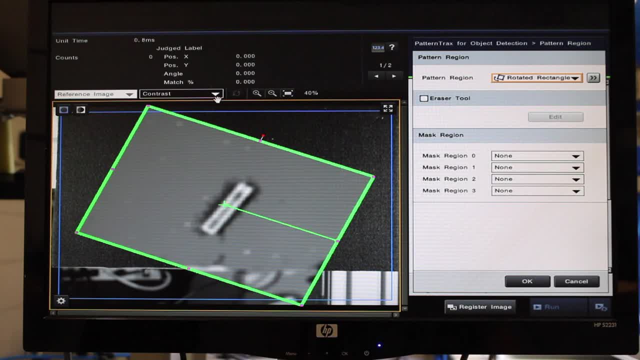 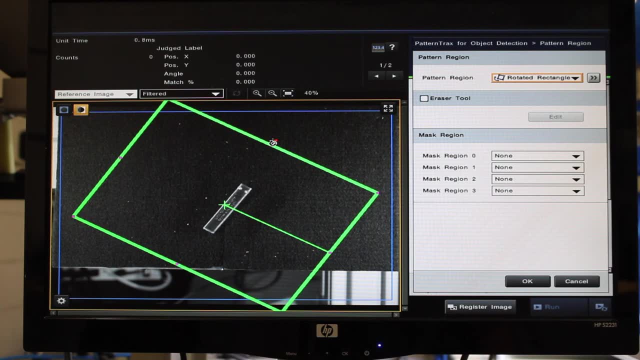 And so here, what we're going to do is we're going to set it up so that we can perfectly outline the piece we are looking for. So we'll grab the corners here and we'll bring them in. We're going to want to give it a little bit of room to breathe. 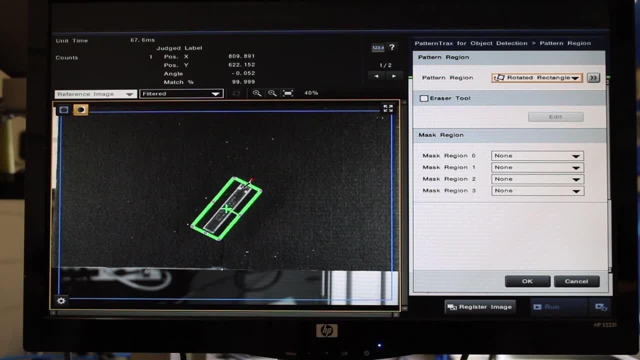 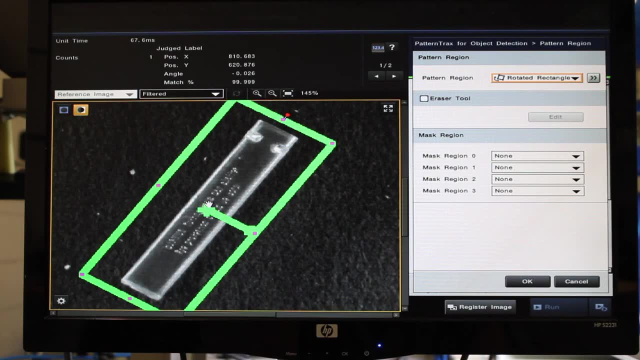 So that way we're not running into other pieces in case they're in close proximity to one another. And so this way, now the system knows what it's looking for. Now we want this embossing to be right side up, But we'll get to that in a little bit. 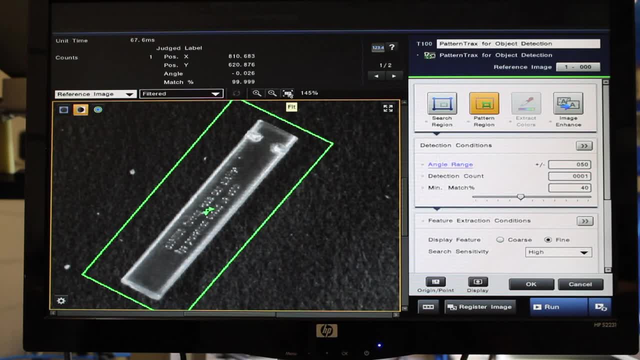 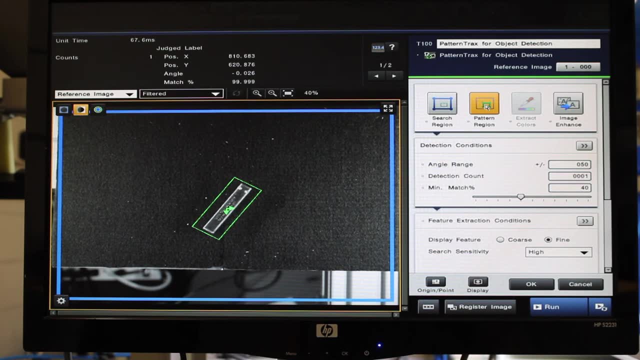 So we'll click okay there. So now the system knows what it should be looking for, It knows that this is a good pick, And so next, what we're going to do is we're going to apply some filters so we can better extract some of the features of our pattern. 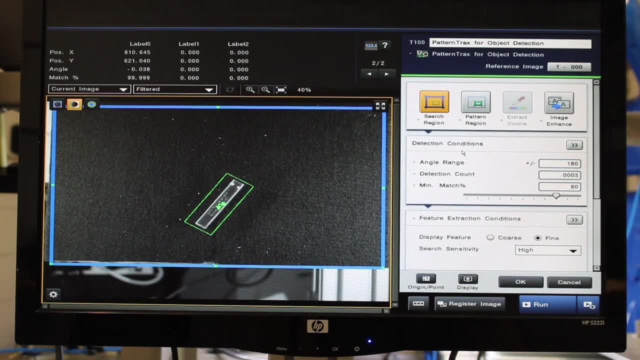 And now we're going to be trying to enhance the image with filters that are available in the Keyence program. So what we're going to do is, up here you see four different options: Search, region, pattern, region, extract colors, image enhance. 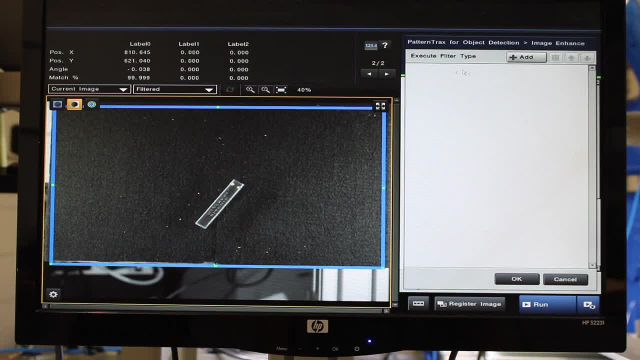 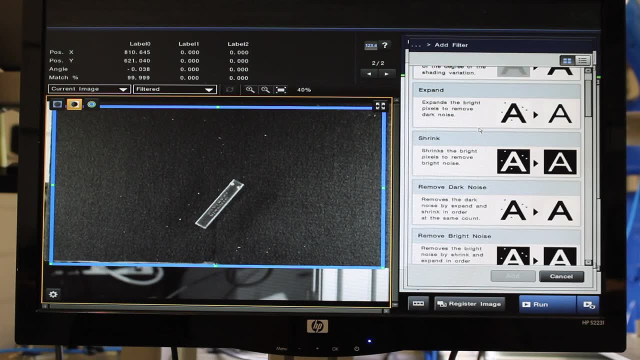 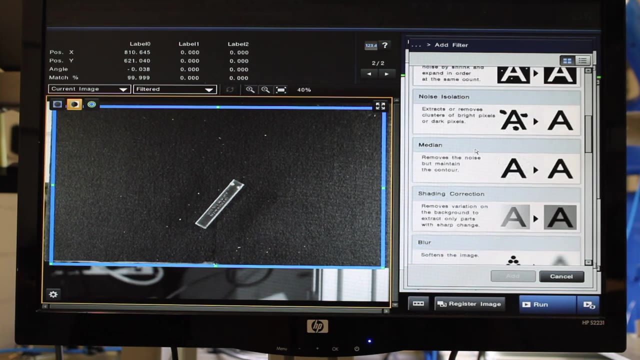 We're going to want to go to image enhance And you can see execute filter type. So all we click is add And we have a list of filters For all types of different purposes. We're going to be using two that I've found to work really well. 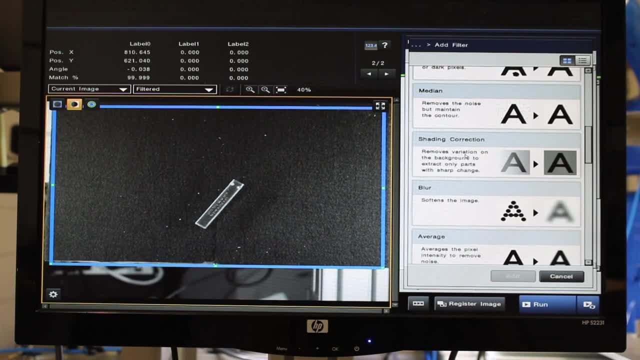 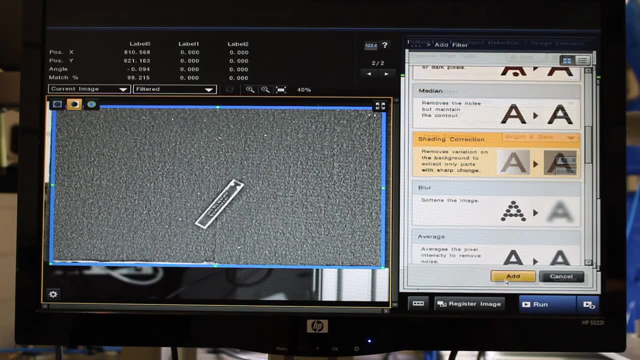 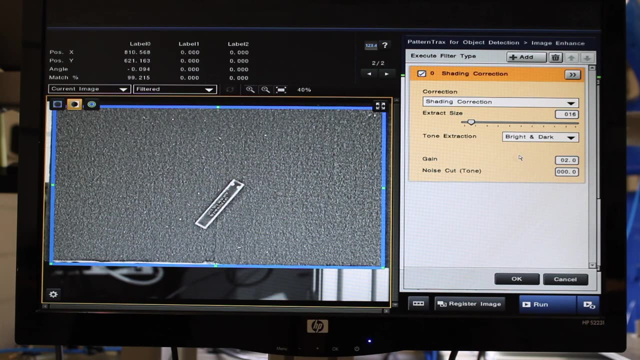 We're going to be using shading correction, Which you can see gives it almost a monochromatic finish, So we're going to add that one. And, you see, every filter has its own setting, So you can tweak the filter as well. So it goes really in depth. 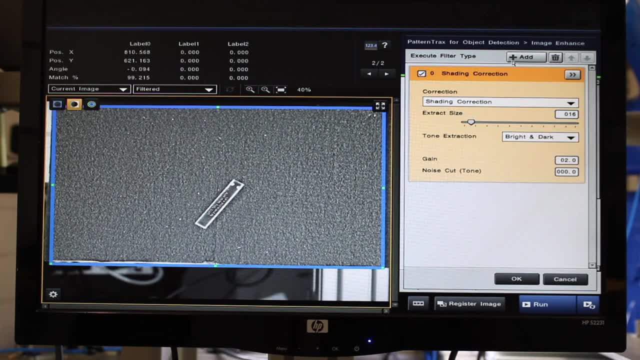 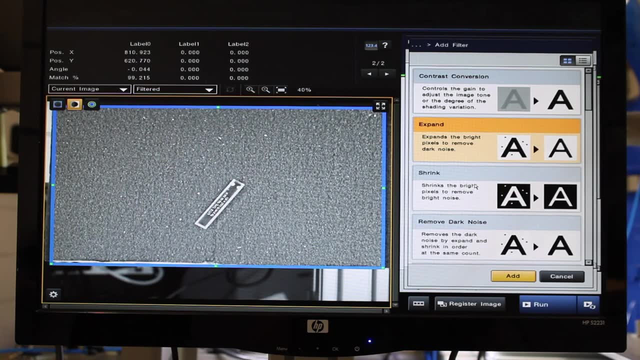 You can do whatever you want to do with these filters, And we're going to add one more expand Which brings out more of the white particles, Because we're trying to bring out the embossing on these parts as much as possible. 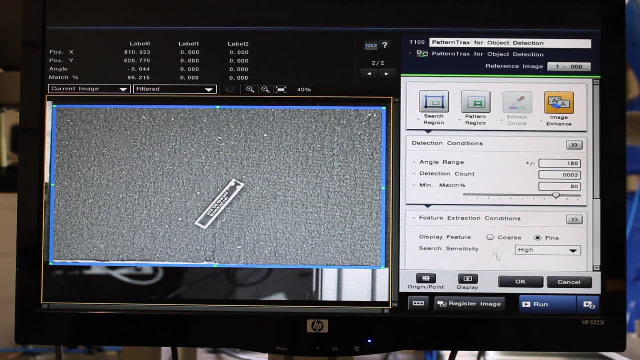 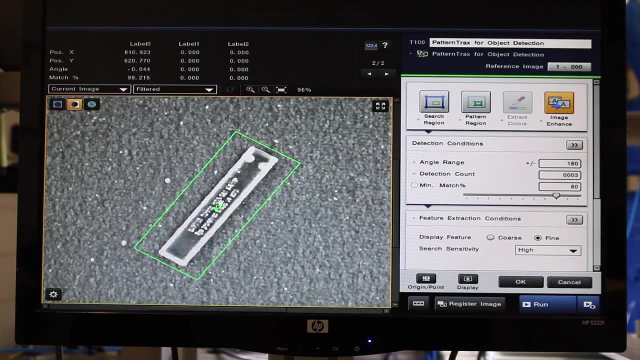 So we'll add that. Okay, You can see, the system still picks it up. It's still picking it, It's still recognizing what we're looking for. It's just we have a more clear image. You see, now it's a lot more defined. 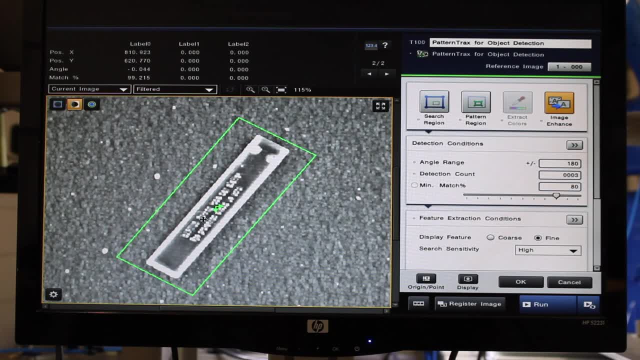 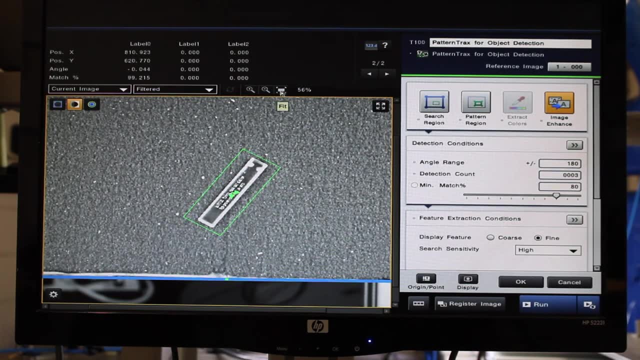 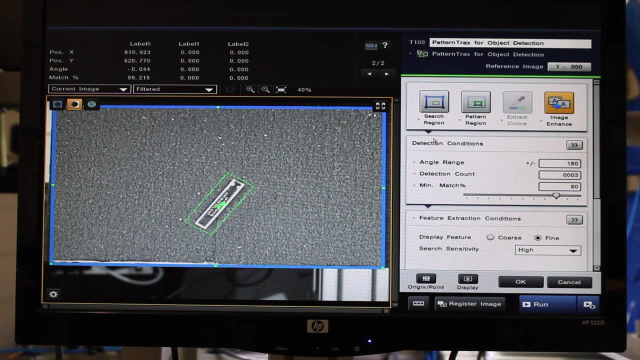 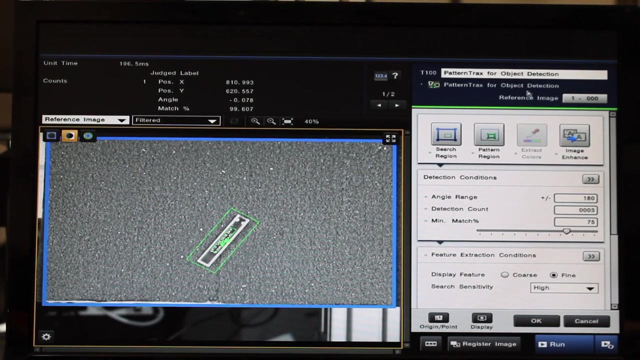 Our edges, our characters. what we're looking for is a lot more defined. So now we Are able to play around with the system using these filters And program it or set it using these filters as the conditions. Okay, So, once you've found the filters that work for you, 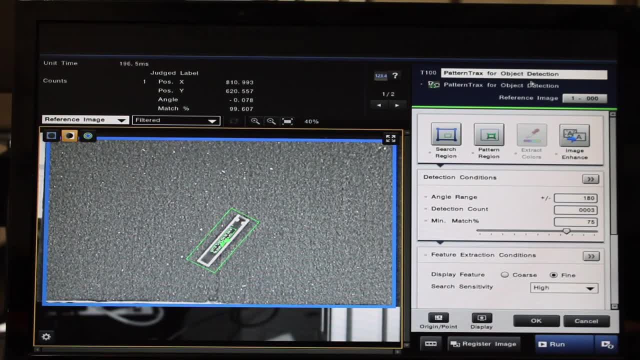 And you've had time to play around with the filter settings And get a clear cut image of what you're looking for. We actually get into the detection conditions. So the detection conditions are conditions That limit the system on what can be detected and what cannot. 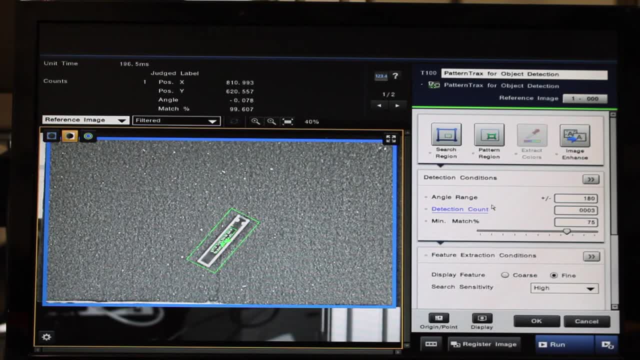 What is a good pick and what is not a good pick. So there are a lot of different detection conditions. You only see three here currently, But we can go further into that. But let me go over these three first. So we have angle range. 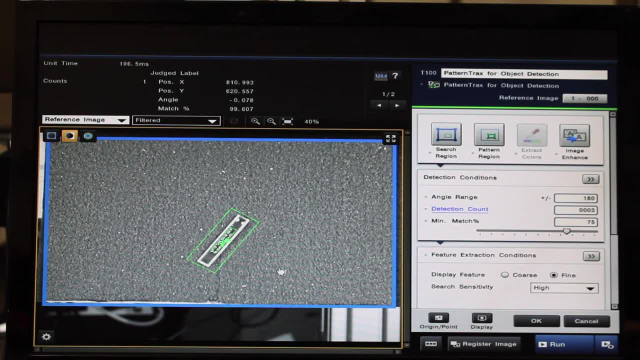 So mine is set to plus or minus 180 degrees, Which simply means no matter which way this part is oriented, The system will recognize it as a good pick, as long as it is right side. up Under that we have detection count. Mine is set to three. 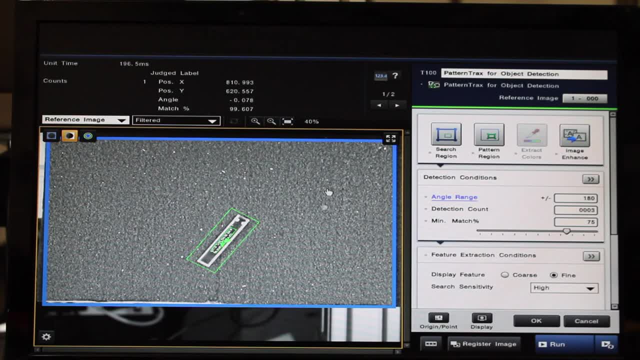 Which simply means that it can detect up to three parts at a time. If we were to set this to one and I had five parts on here, It would only detect one part. So now that it's on three, I can detect up to three parts at one time. 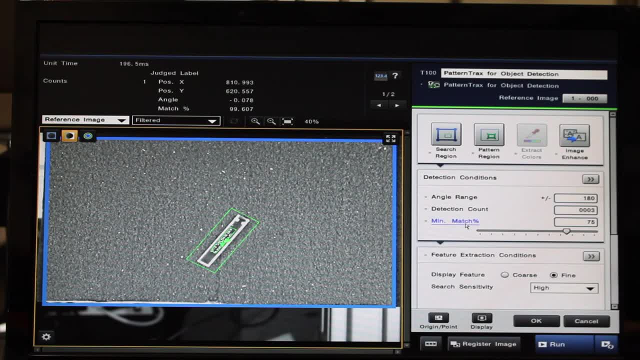 And then I think the most important detection condition here Is the minimum match percentage, Which right now mine is set to 75%. What this does Is it calls to the reference image And it gives a percentage to the current image here. So right now we're on our reference image. 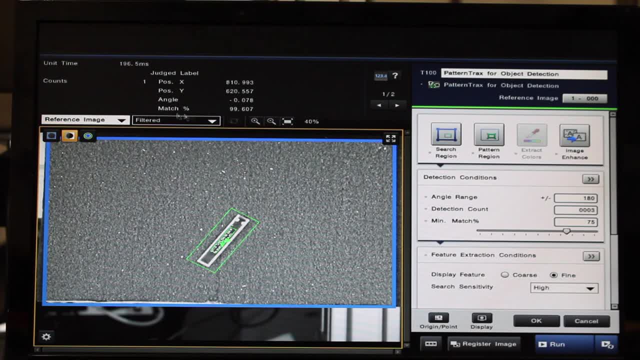 And so you can see that up here. it gives us a match percentage of 99%- 99.607%. So, since I have the minimum match percentage set to 75%, Anything under a 75% match to this reference image Will not be recognized and will not be picked. 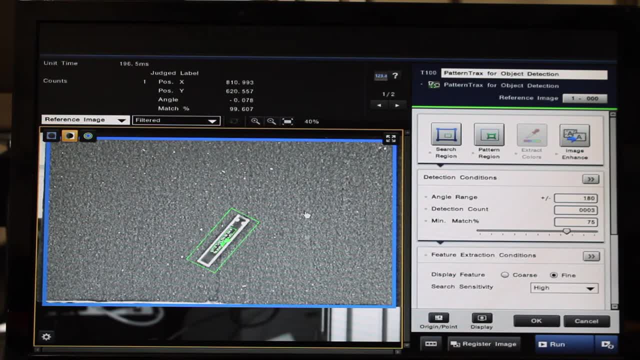 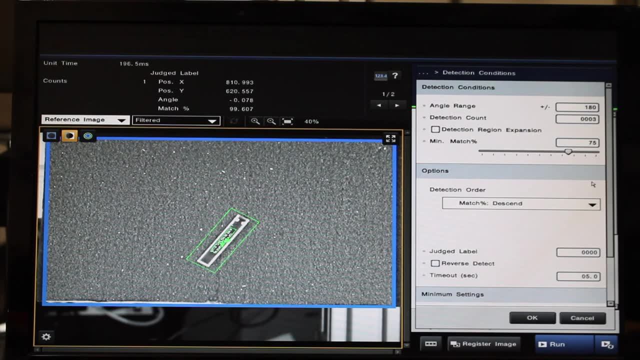 Anything above this Will be recognized and will be outlined by the system. Now, if we go further into detection conditions, By clicking the double arrows up here You can see we have the same conditions we were just looking at, And then we have a few more. 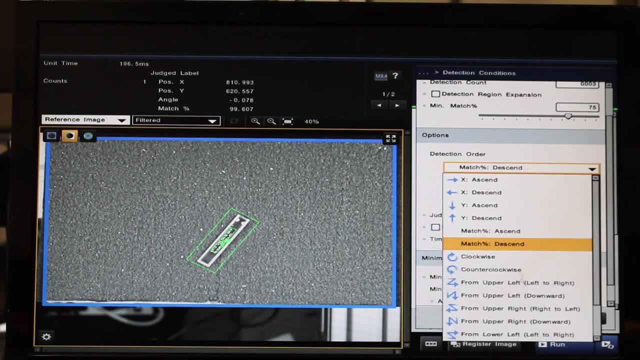 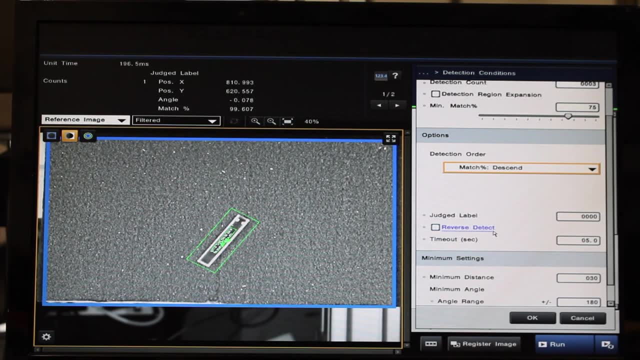 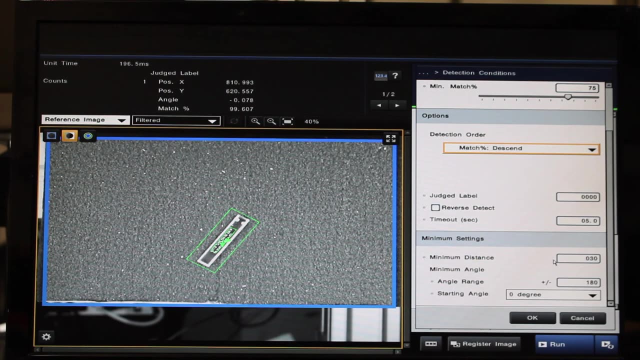 You can the detection order Right. you can change that How it organizes them in terms of detection. We have our timeout in seconds for the program, And then here we have minimum distance, Which is also a very important condition. Minimum distance simply means: 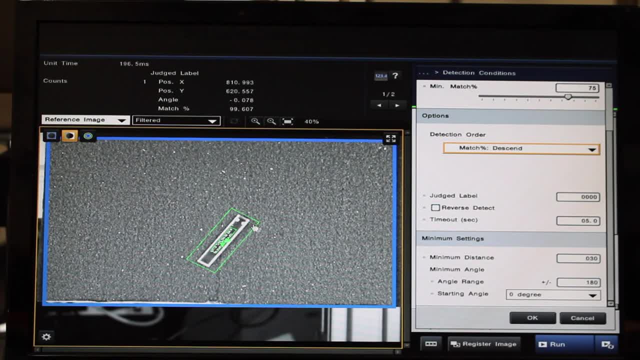 That any parts within 30 millimeters of each other Will not be recognized. So this is in millimeters, So anything within 30 millimeters of each other Will not be recognized, Any parts that are 30 millimeters or more apart. 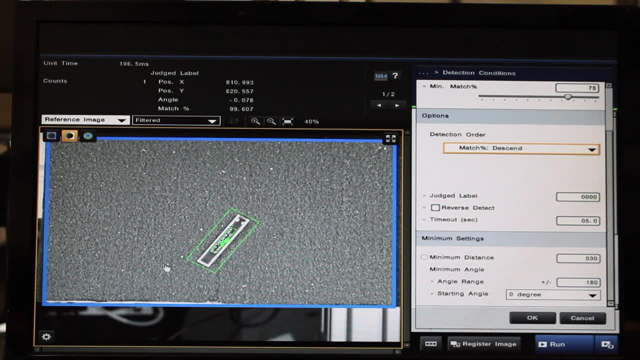 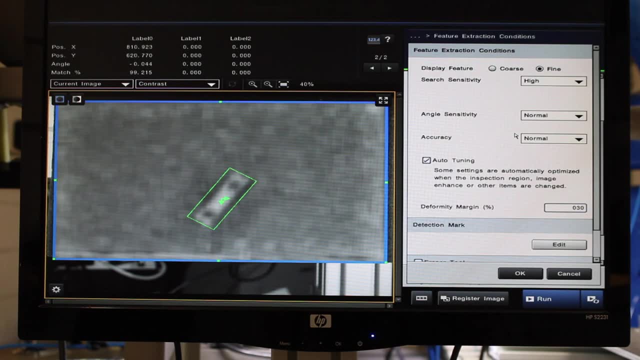 Will be recognized and will be outlined by the system as a good pick. And we have our feature extraction conditions Which we're able to set a. We're able to set a detection mark, Which is what we're going to be playing around with. 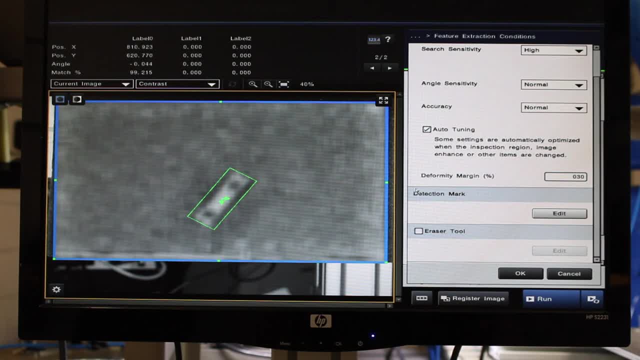 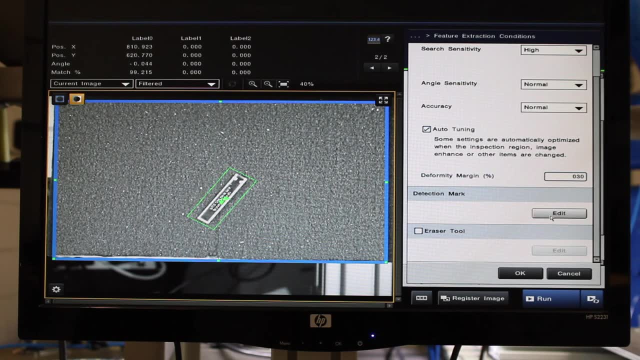 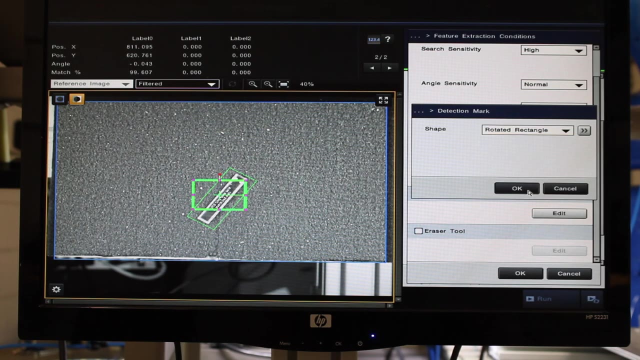 So the detection mark Tells the program To search for a certain mark or feature On the part. So if we set a detection mark And we can choose the shape again, We're going to do rotated rectangle And what we're going to do is we're going to rotate that. 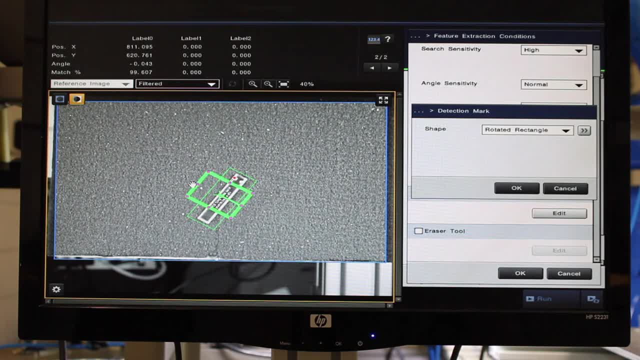 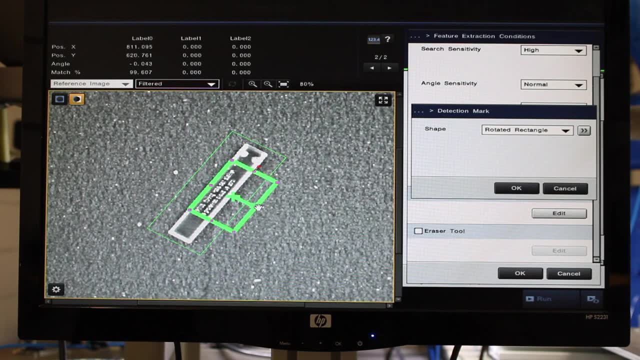 To embody our lettering, Because what we want on this part Is for the lettering to be face up. We want it to be picked in this certain orientation, With the lettering or embossing face up, So that it can be placed in a certain orientation as well. 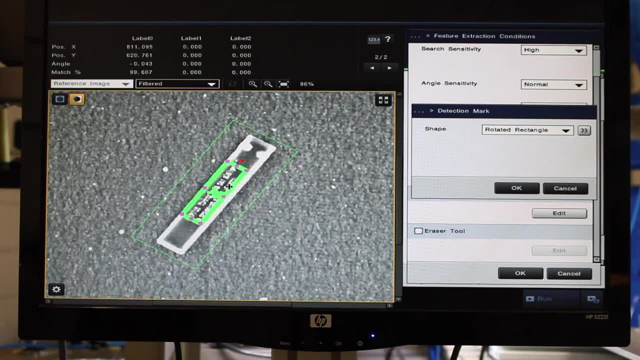 So what I'm going to do is I'm going to take the detection mark And I'm going to make it hug the lettering As tight as possible. We don't want to get any of the outer edges in there, And so now we have the detection mark. 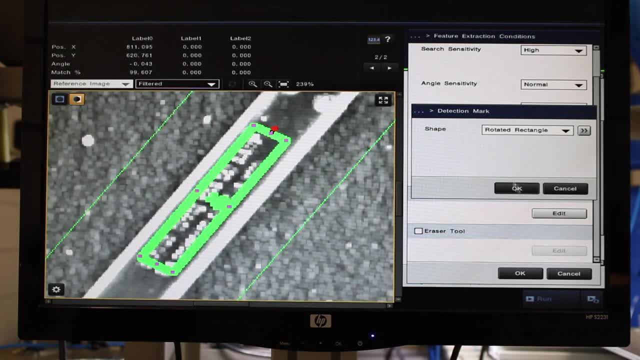 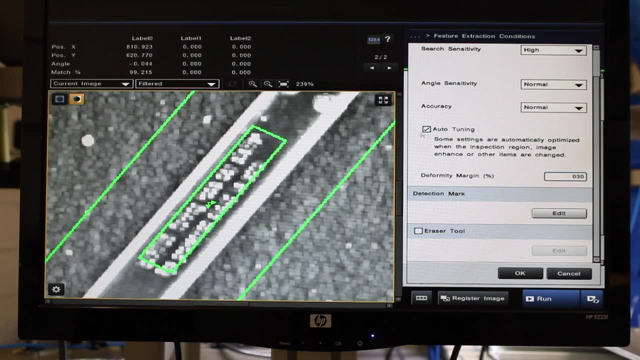 Looking around our embossing right here. So we'll click okay. And now what you can do Is you can actually set the feature extraction size. So if we uncheck this auto tuning, You can see the feature extraction size in pixels. 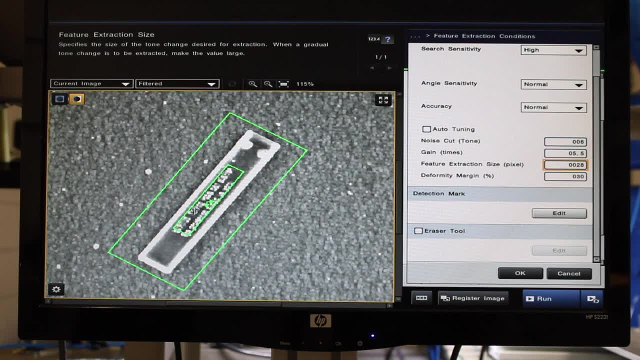 And so what that's doing is, Once a certain amount of pixels are detected, It'll show that as a good pick And it'll pick it. Anything less than that And it will not pick, And it will be registered as no good. 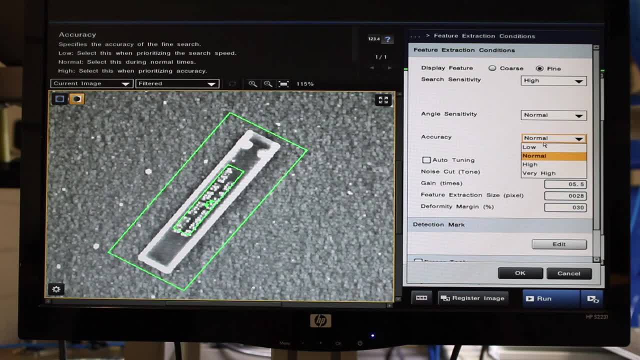 And so that's something that we really want. As far as accuracy goes, I'm going to change it to high So that we have a better chance of getting correct positive picks, Because we don't want any false positives or false negatives, And we'll go ahead and click okay, there. 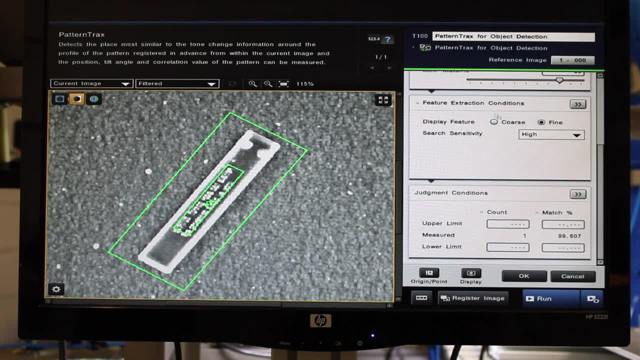 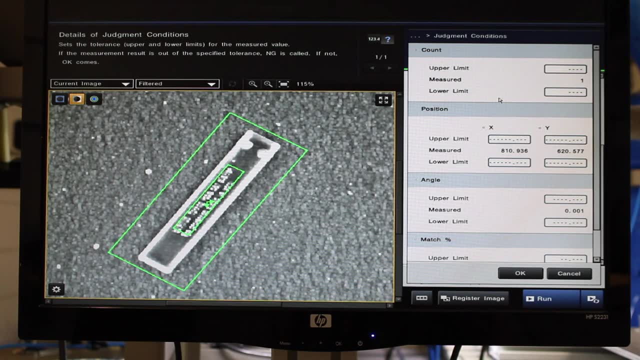 And then you also have, of course, judgment conditions. Which judgment conditions are Conditions on whether or not it will be a good pick. This is same as detection conditions, in fact It's just a little bit more in depth. So you have count: upper limit, lower limit. 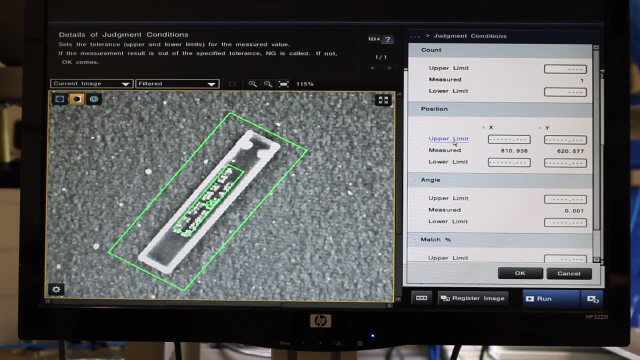 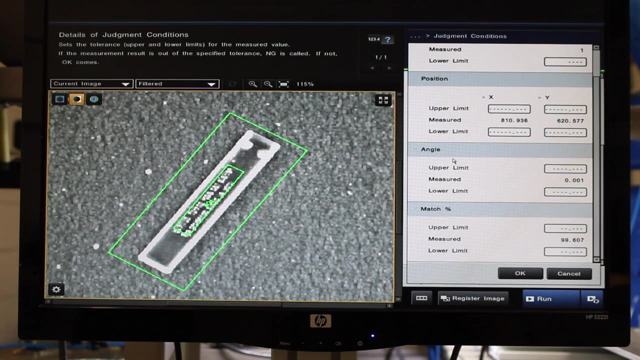 How many it's detecting Position. You can set an x- y position. So if it's outside of a certain x or y position, It will not be registered as a good pick. You can set an angle limit. Your limits are 30, positive, 30, negative, 60.. 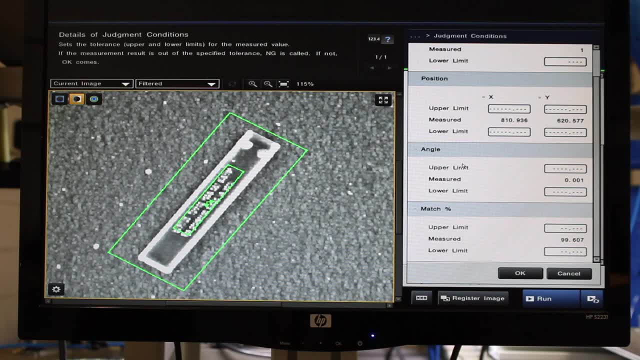 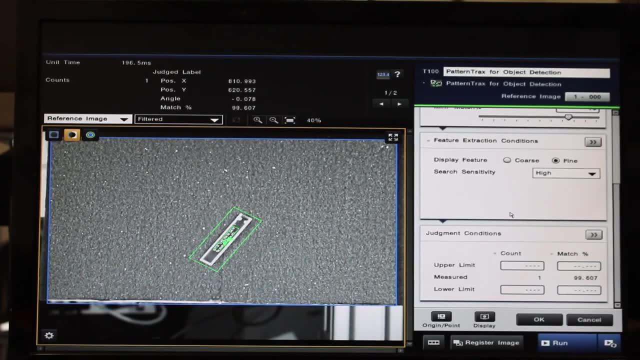 You can set that here, And so anything outside of that range will not be picked. And then, of course, match percentage. You can set a lower limit and an upper limit to match percentage. So once we're done with all the feature extraction conditions. 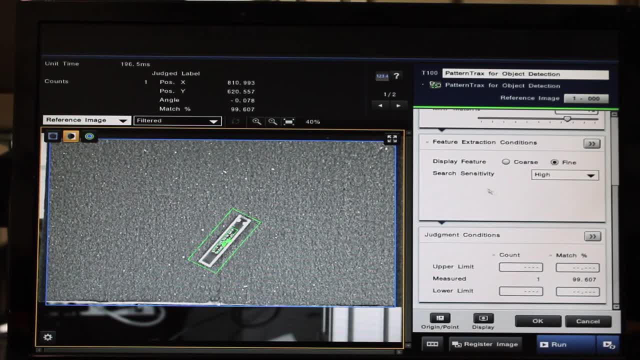 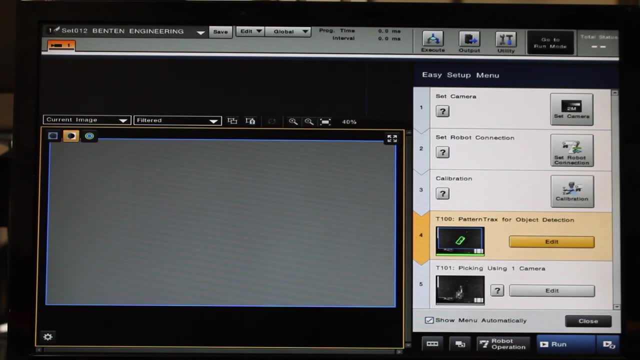 And the detection conditions, And once we're able to confirm that the system is correctly picking these parts, We're done with pattern tracks And we can move on to the next step, Number five, Which is picking using the actual arm, And so I already have this set up. 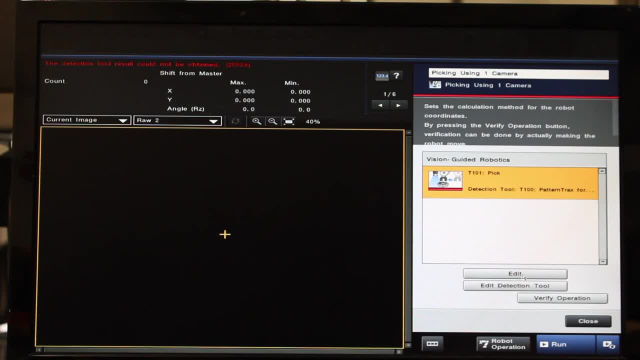 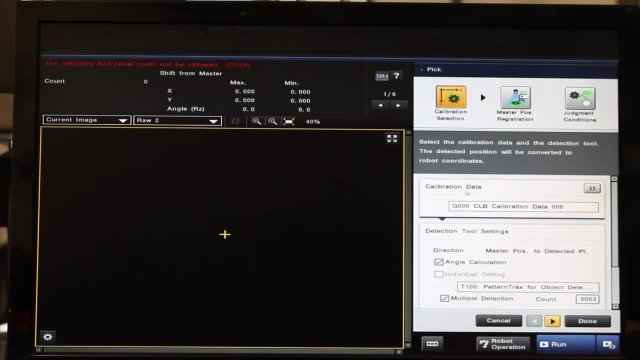 If we go into edit here, If we go into here And we can go into edit, And so you can see, we're calling the calibration data from earlier, before The calibration data that we set up. We're calling that And we're also calling the pattern tracks for object detection that we were just working on. 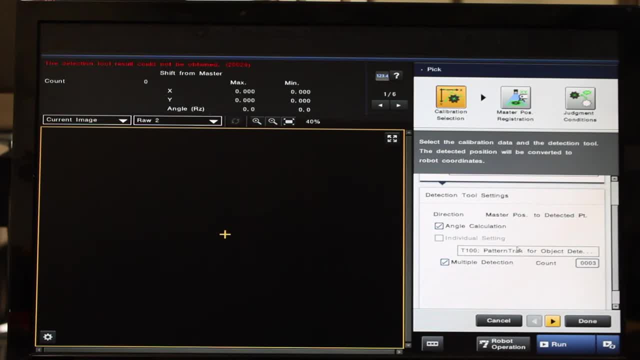 So it can pick the correct parts And call for the arm to come down and grab them. The one thing we do want to tick is multiple detection. Now, this is circumstantial, But for our circumstance we want to be able to detect multiple at once. 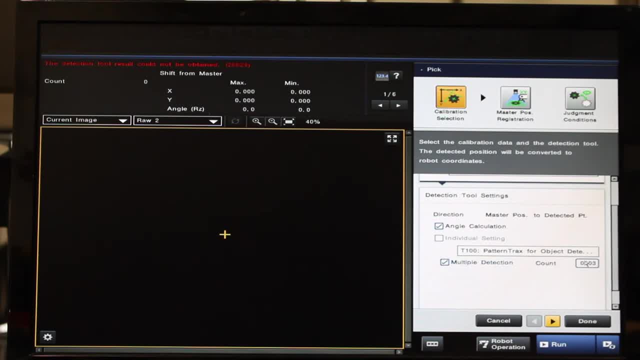 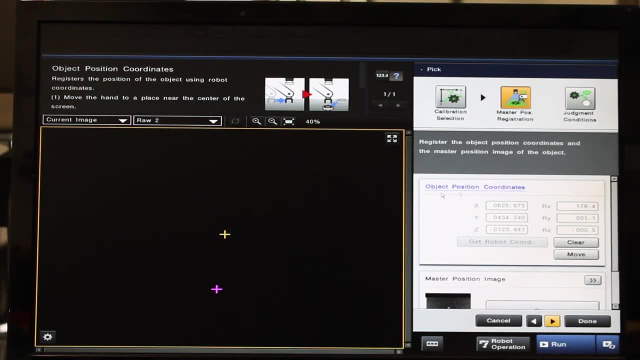 And so we're going to click multiple detection And I have it set to three again. Once that is done, we can head to the next part, And the next thing we want to do Is we want to set the object position coordinates. So what we're going to do is: 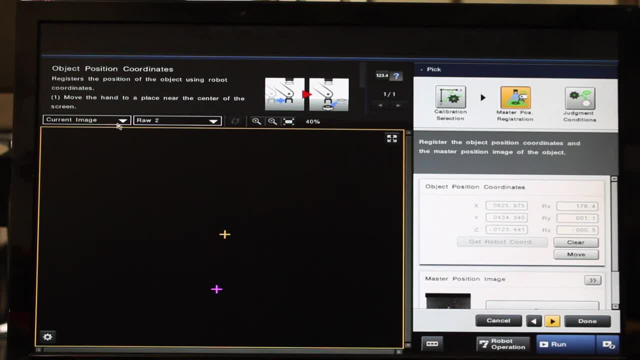 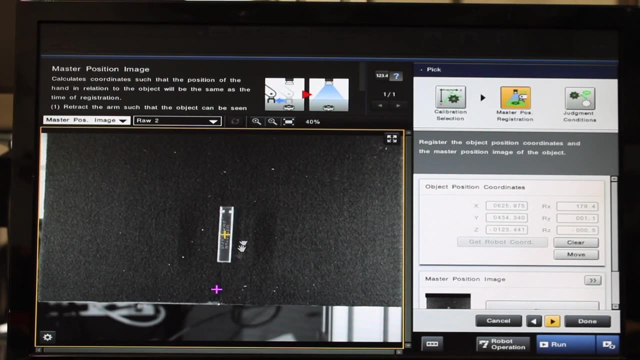 We place the object or the part that we are wanting to pick, We place it in field of view of the camera And then we'll bring the robot arm down exactly how we want it to pick that item. So, as you can see, we have our parts in the correct position that we want it to be picked. 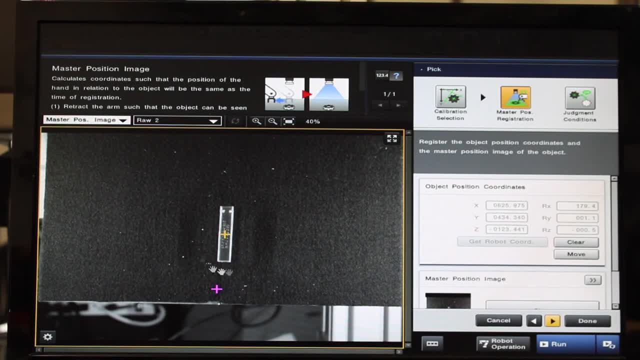 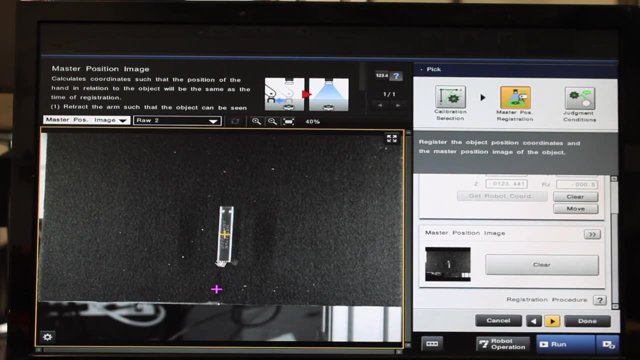 And you can see we have a little yellow cross, Which means it is being picked up by the vision system, And we have the position coordinates already set up And our master position image is set as well. This is our master position image, Which is simply a reference image for our picks. 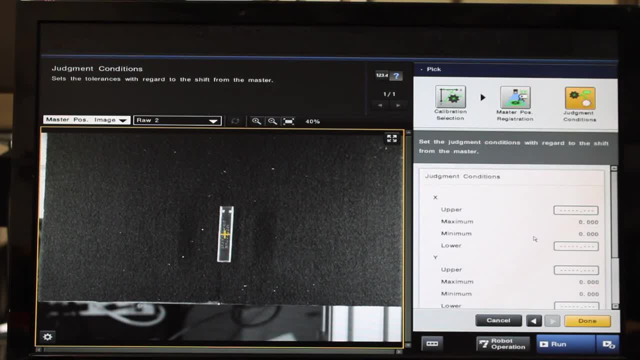 Once that is done, we can move on to our judgment conditions, Which is different from our detection conditions. The judgment conditions are judging whether or not the arm will pick this or not, So you can set an X, Y and a rotational angle limit. 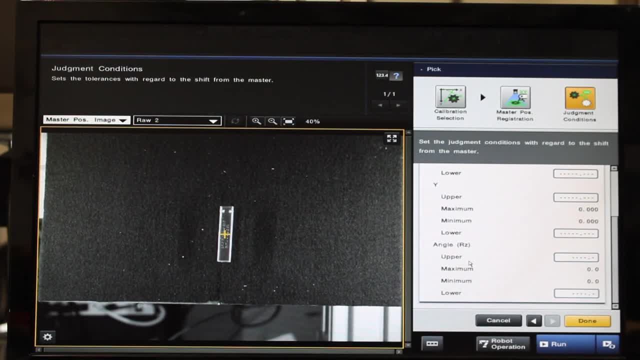 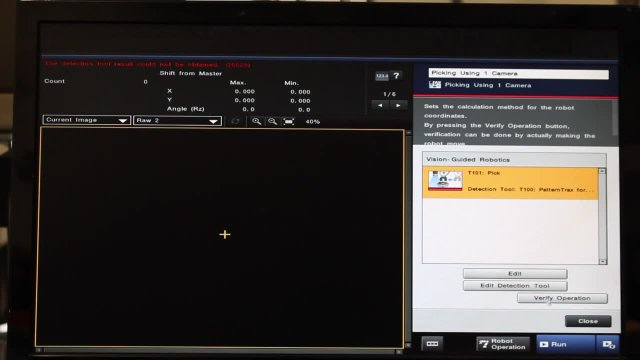 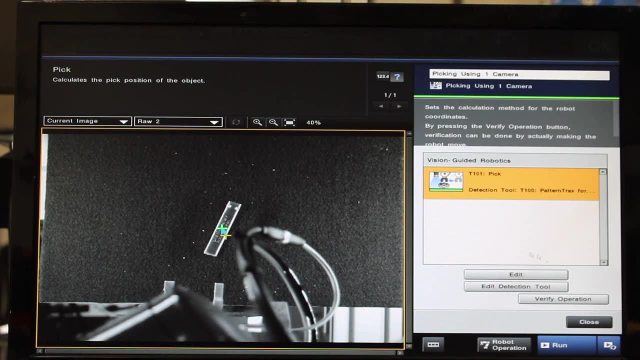 So anything outside of those limits will not be recognized And will not be picked. And so once we are done there, We are completely done and we can move on to verifying the operation flow. Now we are going to verify the operation of the arm. 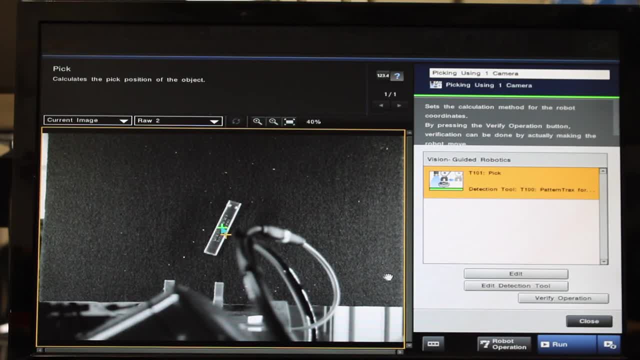 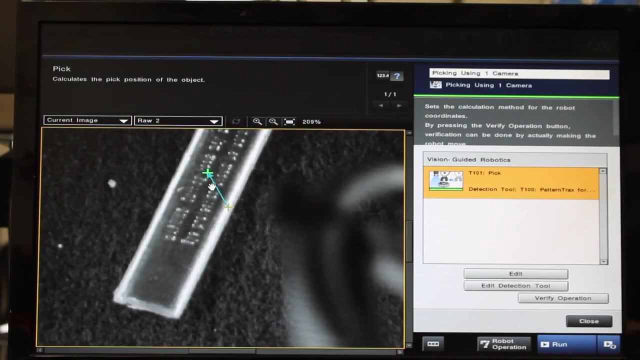 And make sure that it is picking correctly and accurately. So I currently have one piece out here And the vision system is picking it up correctly And it is calculating the path to the object. Now we just need to make sure that the Robot is able to pick it correctly.